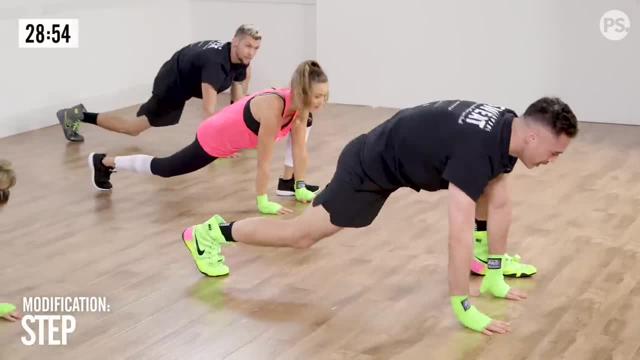 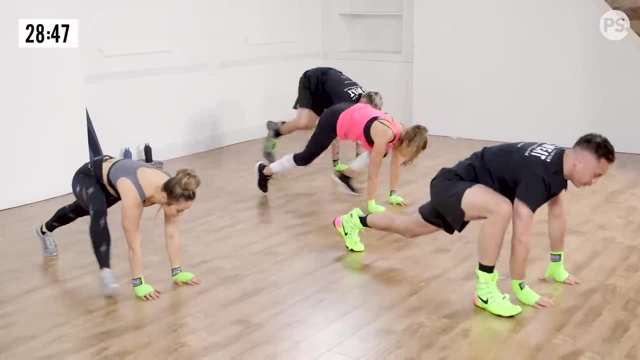 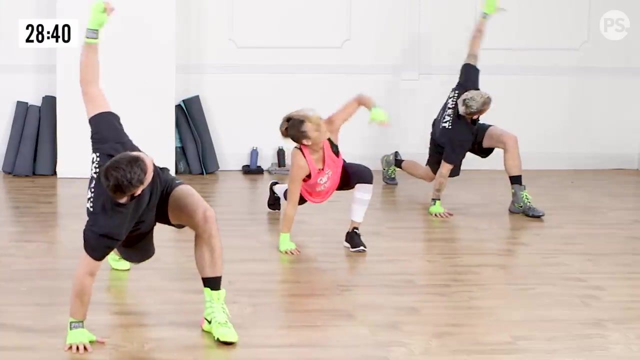 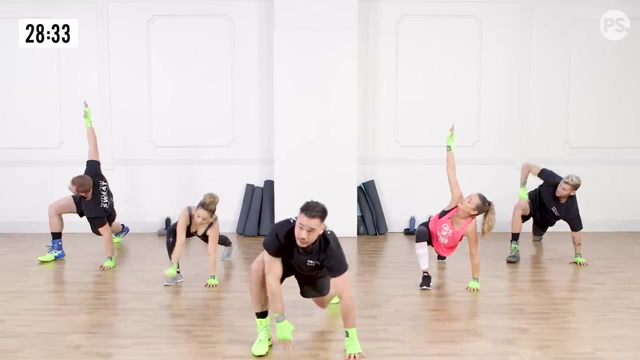 three mountain climbers. So one, two, three And we're going to rotate up towards the ceiling Hold for three, two. one Hand goes back One, two, three. Other side, Good Hand goes back One, two, three, Rotate. And one more: One, two, three And rotate Good guys From here. 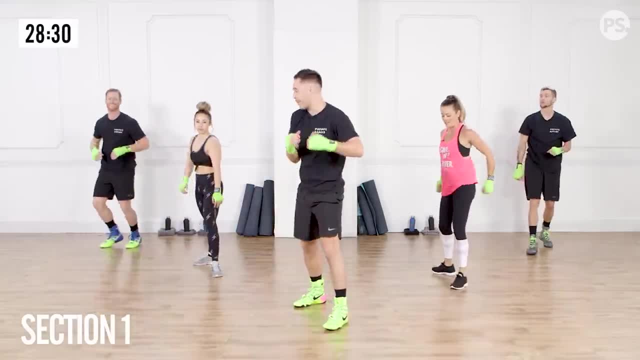 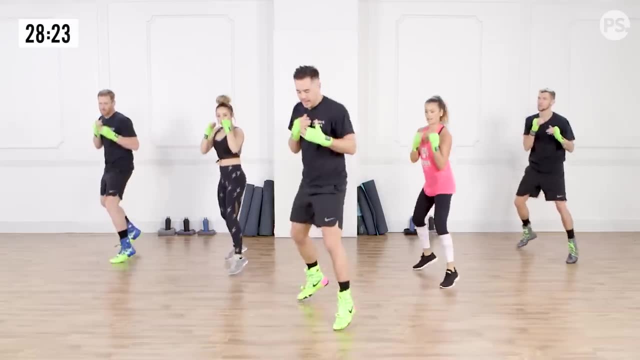 back up on your feet. We're going to go into what we call the prevail bounce. All right, Yeah, So from here I'm just pushing from front foot to back foot. I've got my left side forward And since today's going to be a boxing workout, we're going to keep our hands up. 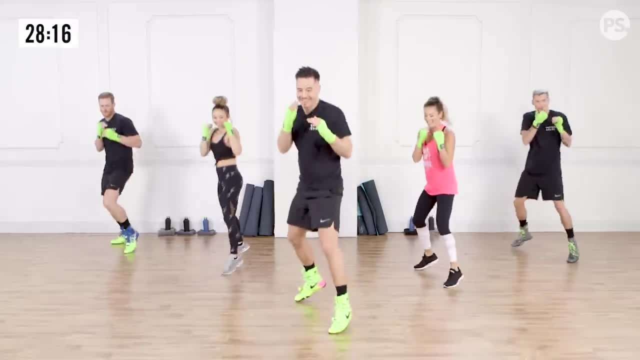 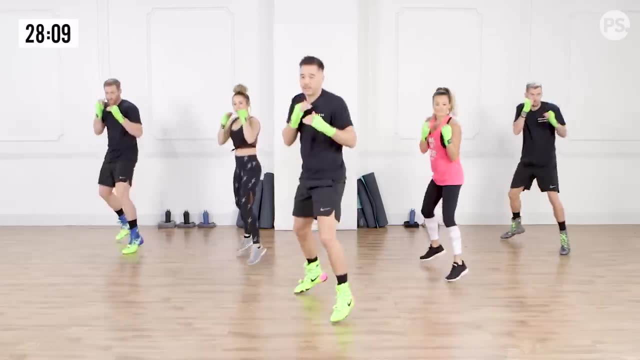 nice and high. Make sure we protect the moneymaker. like that. There you go, Good Nice guys Going forward and back Few more seconds. Start to feel the calves here a little bit. Milan Feels good. 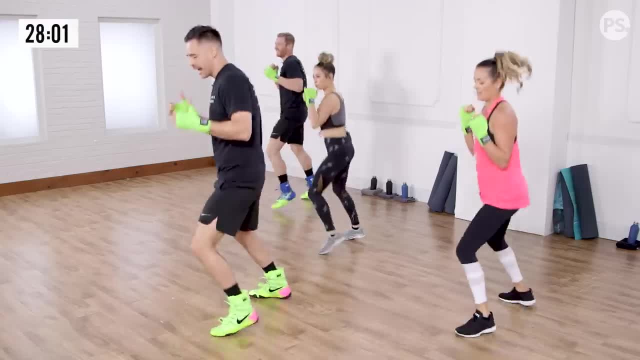 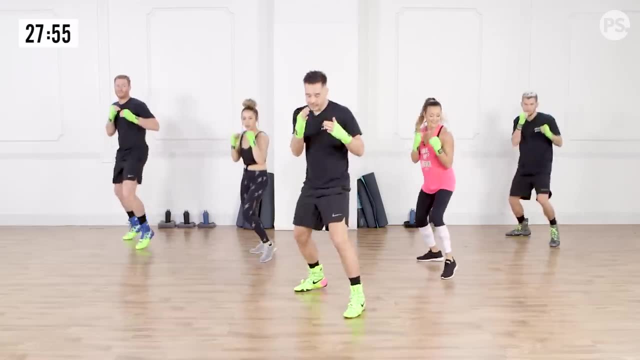 Yeah, So it's important in boxing that we have this nice bounce. This is actually where we recover in boxing. okay, So from here we're going to plant our feet. We're going to keep the left foot forward, right foot in back. You're going to pick up your right. 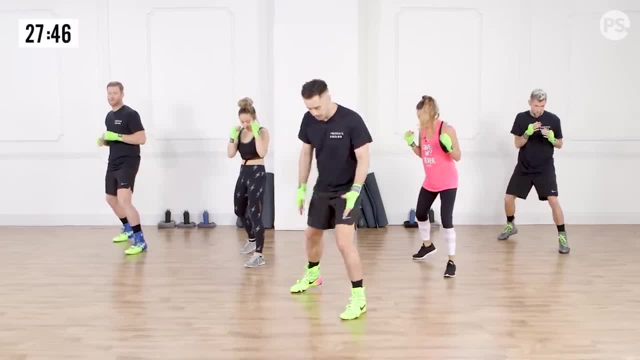 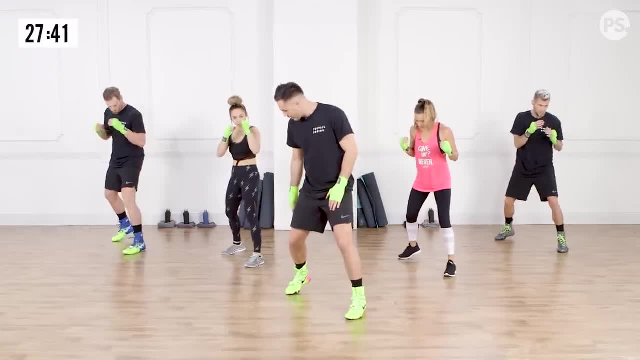 Stagger, Staggered, Staggered, Staggered, Staggered, Staggered, Staggered, Staggered. I don't want my feet in alignment going this way, So I'm going to step out to my right- my right heel off the ground. 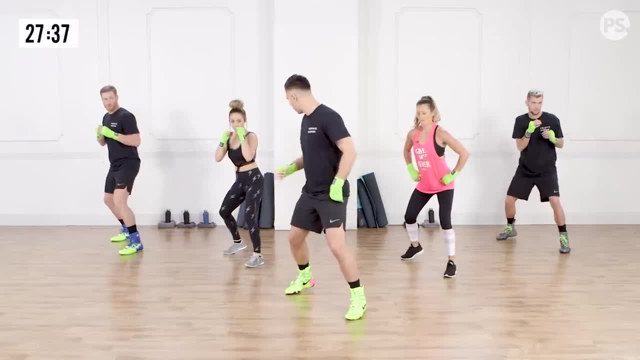 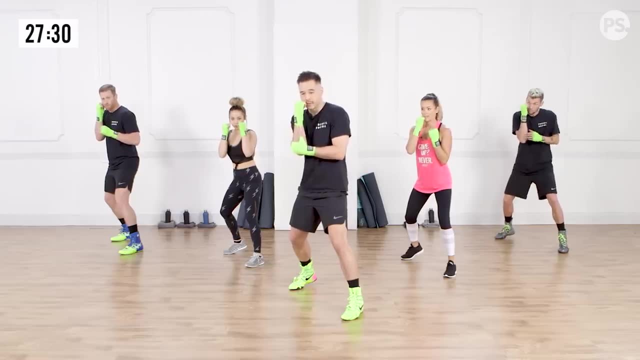 and I'm going to push my hips back like I'm sitting into a chair. Awesome, Very nice guys. From here, right hand's going to come up touching the face. arm is against the body. This is our shield. Left hand it's going to be out front. So this is our first line of defense. second line: 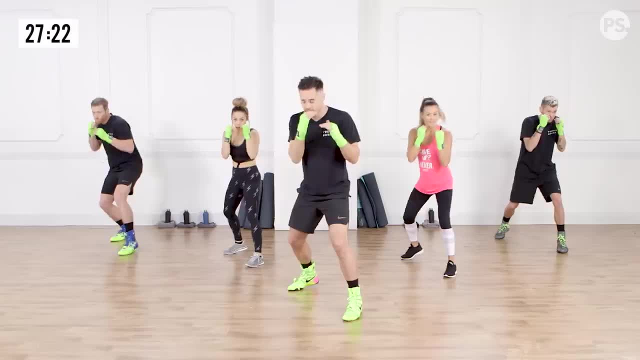 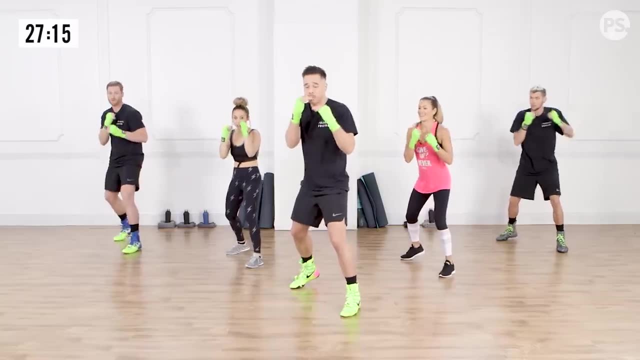 of defense. From here we should be bouncing up. where we can move our head, We can step away, step in and, most importantly, we can throw all our punches. All right. So first punch that we're going to learn today, guys, is called the jab. It's our left hand and it's going to go straight. 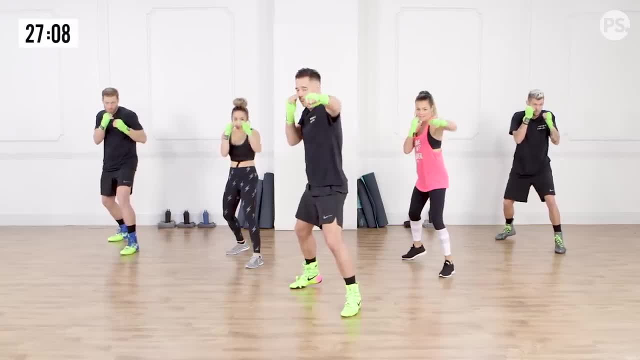 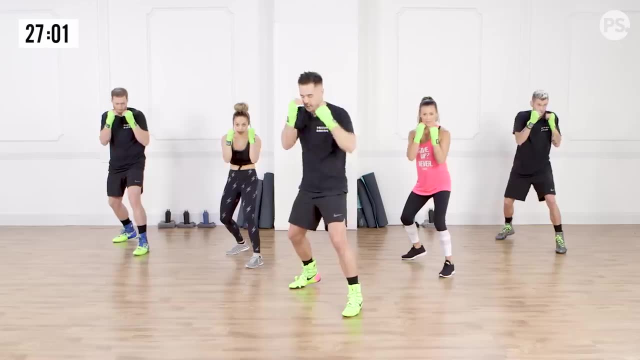 out and come straight back. You'll notice that when I throw this punch, we're rotating the fist and also getting rotation through my shoulders. All right, So this is our jab, also known as the one. All right, Straight out, straight back. Good, Now, when I say go, I want you guys to throw the. 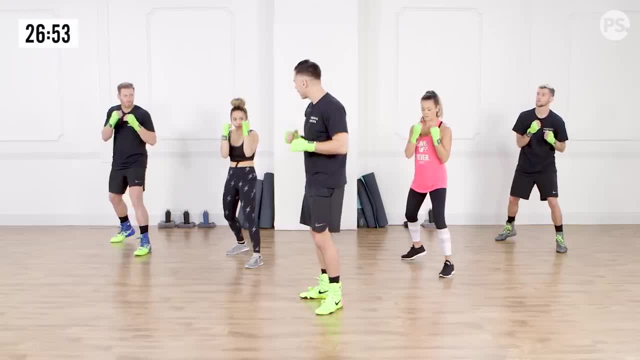 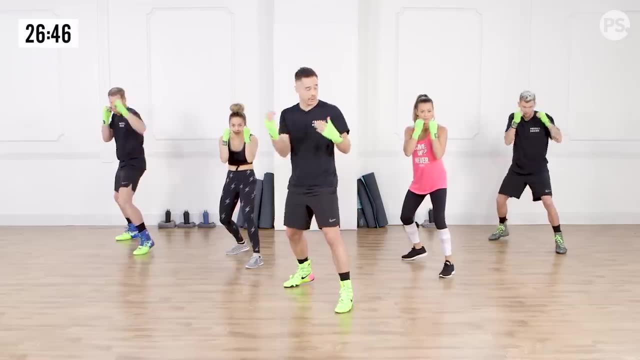 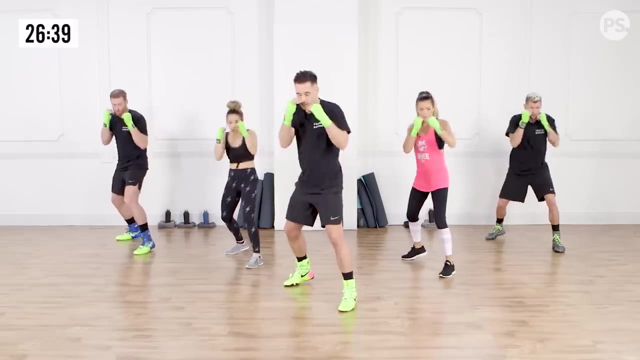 jab Not too hard, just out and back, keeping the back hand up, Ready And go, Go Good. And straight back to the chin, Go Good. And so they're already doing this, A nice little exhale with each punch. So you're making that noise And back, Ready And go, Good Go. 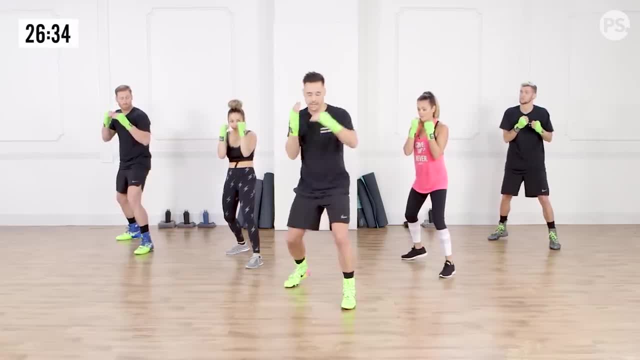 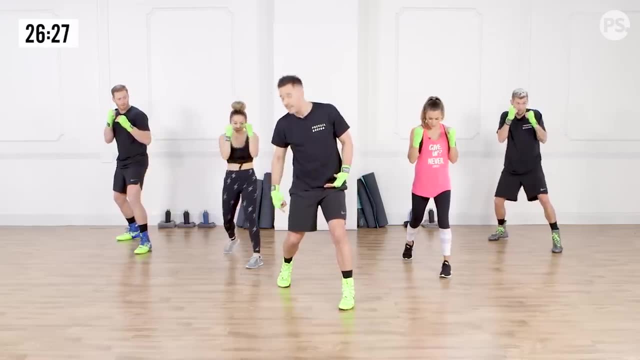 Nice. Second punch that we're going to learn today is the cross. It's going to be our back hand, So we're going to go straight out and come straight back to the chin. You'll notice that when I'm throwing this punch, I'm rotating my hips and pivoting my back foot, All right. So. 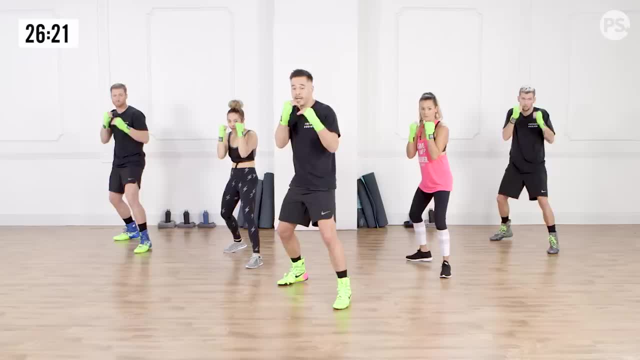 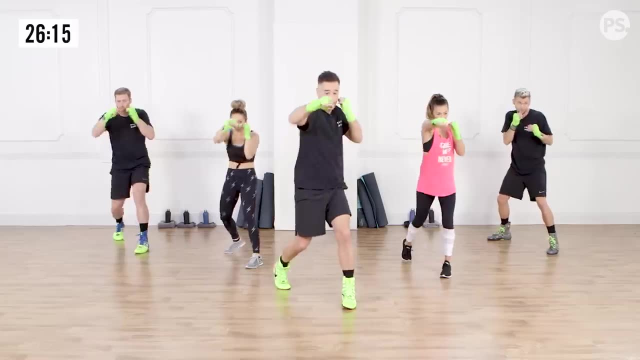 we're going to punch straight out and straight back to the chin Ready And go Straight out straight back, Nice and easy, Focusing on good technique, All right. So the goal for this portion is really to progress in our knowledge. We're not looking for perfection. 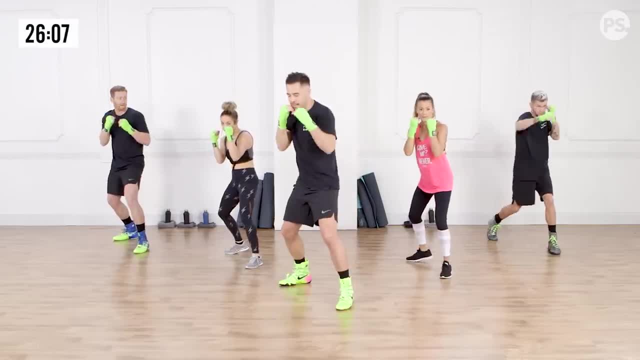 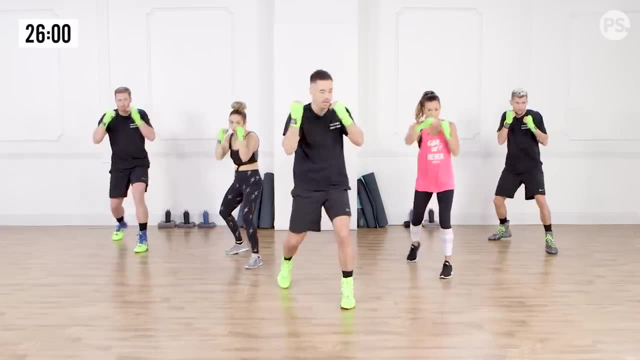 We just want to get a little bit better with each rep. Okay, Hand, coming back to the chin, rotating the hips, Make sure that you guys feel nice and balanced, Ready And go And back, Go And back. So in boxing there's a number system: The jab is the one, the cross is the two. So we've 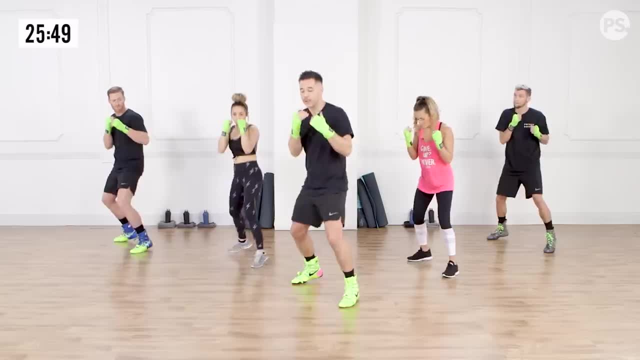 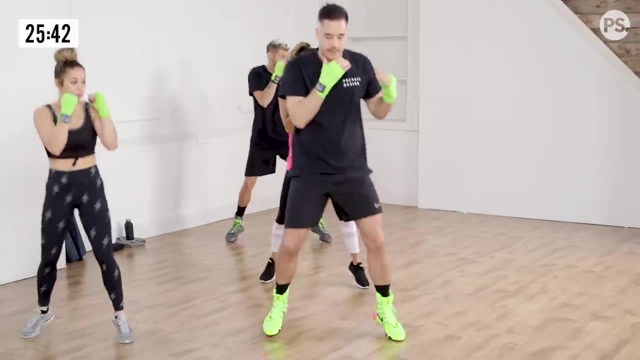 got the jab cross. So when I say, go, I want you guys from the bounce, you're going to plant your feet and you're going to throw the one, two, And after you throw the one, two right back to the bounce, All right. So this is where we're at: Ready And go, Plant the feet One, two, Right. 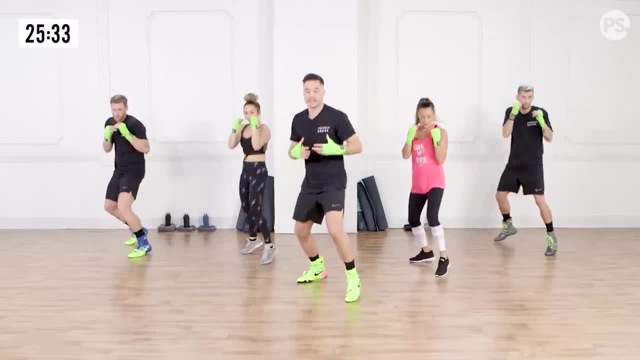 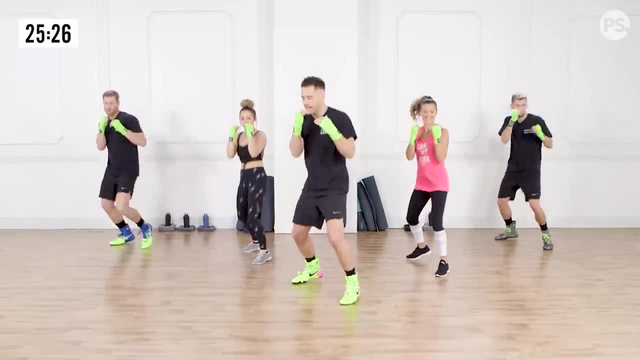 back to the bounce Hands. stay up. Core's engaged. Core engaged means I'm flexing my abdomen And this is what I'm activating as I'm rotating and throwing these punches. Okay, Ready And go Jab cross Good. 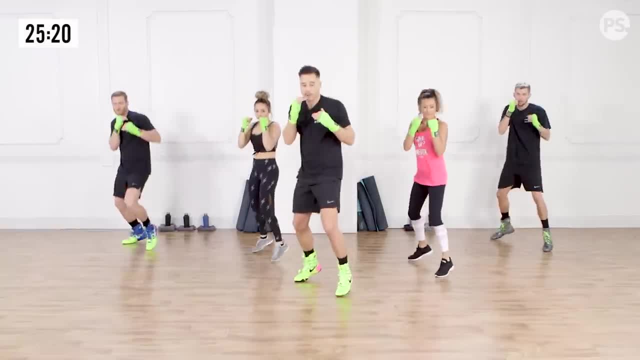 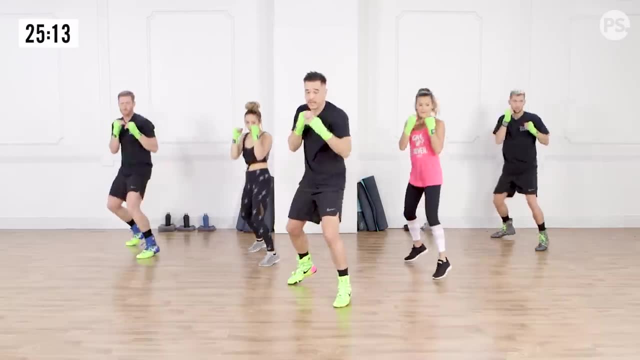 And go Good All the way out. Make sure you guys are rotating your fists And go Good, And go Good. So now, guys, we're going to add a progression. All right, Leilani, here she's going to be. 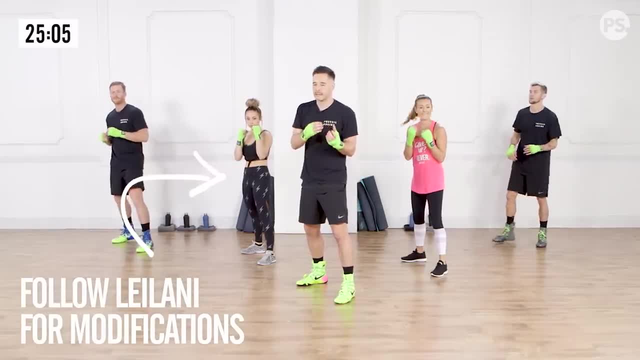 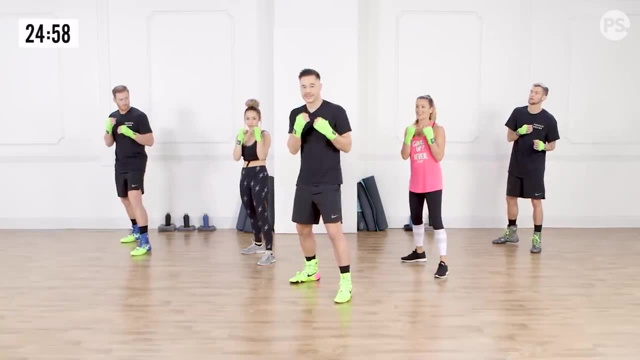 modifying a lot of the exercises that we do, So if you need an alternative that's a little bit more simple, please feel free to follow along with her. For the people that want to take it to the next step, we're literally going to step forward. As I throw my jab, I'm going to step with my left foot. 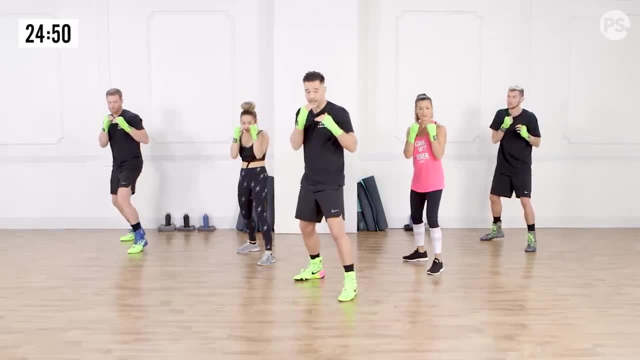 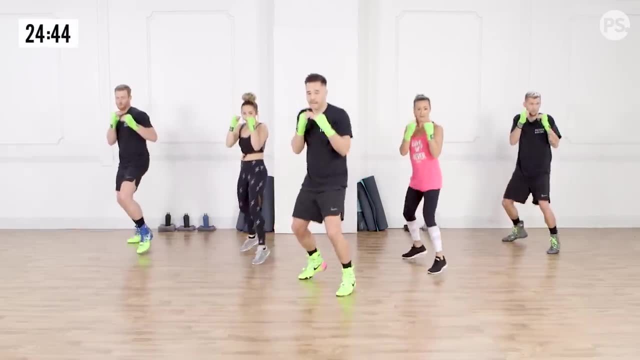 I'm going to step with my right foot, Reset And step back, All right, So we're bouncing And go Step, Step, Reset- Good Bouncing, And go Step, Step, Reset- Excellent. So in boxing, a lot of. 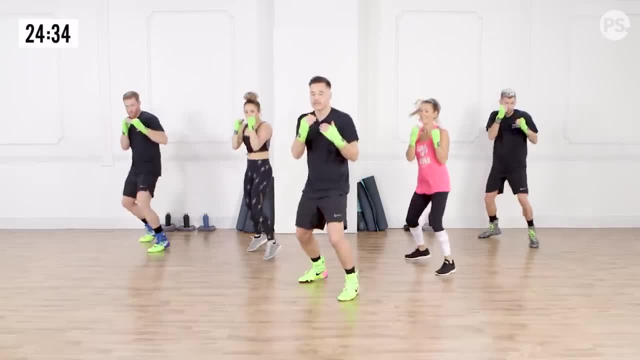 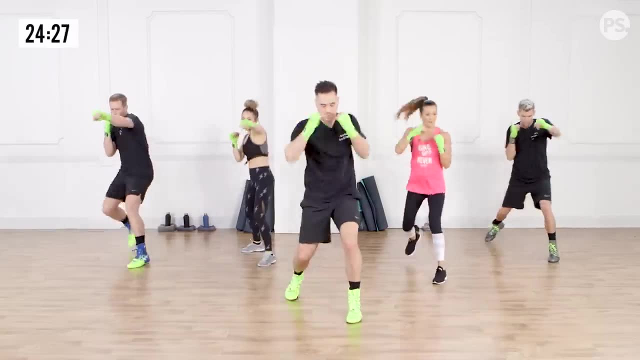 times. our opponent isn't going to stand there for us to hit them Right, So we've got to coordinate our hands and feet together to chase them down And then reset All right Ready And go One, two And back. Good Go. 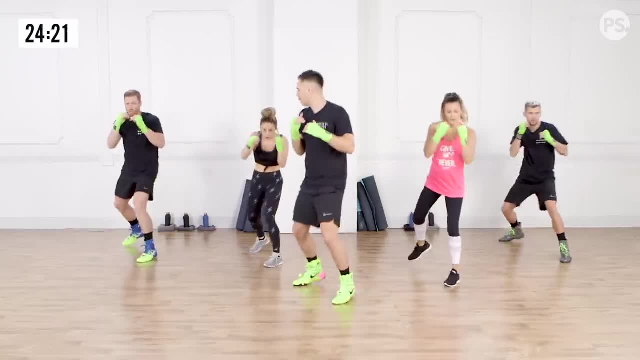 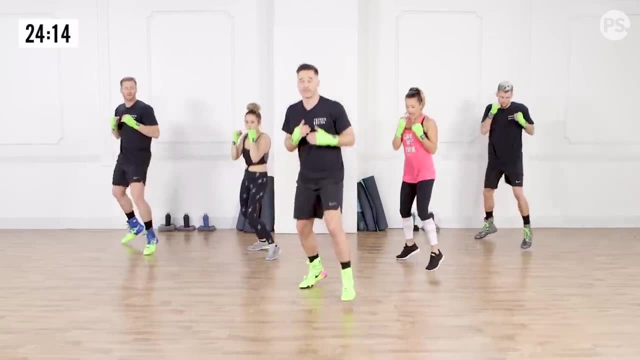 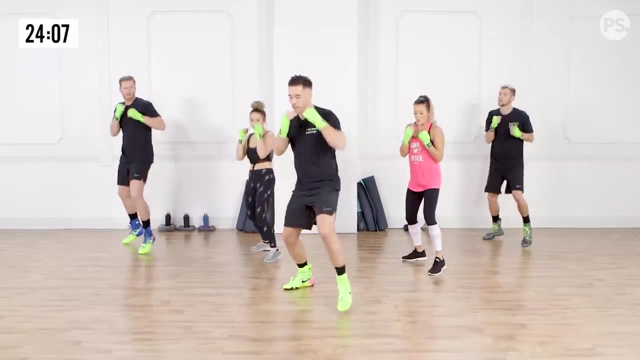 And back Nice. Go Excellent, Go Good, Make sure that you guys are rotating that back hip, because that's where we're generating the power for the punch Ready And go Nice. So now we're going to take it a step further And we're going to go four punches. So I'm going to go one, two, 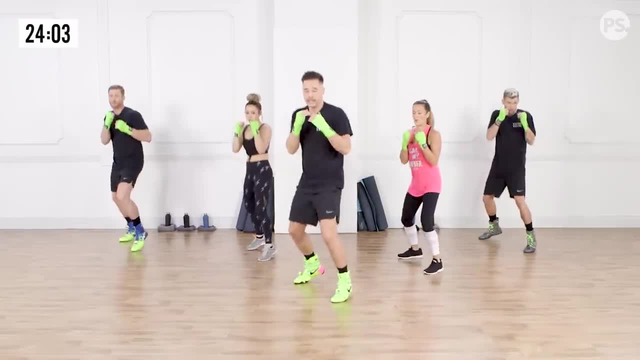 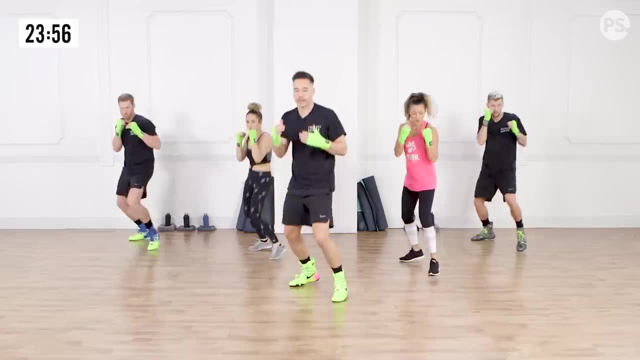 one, two, And then I'm going to reset Ready And go: One, two, One, two, Reset, And again we're focusing on progress. So every repetition that we do, we're just trying to get a little bit better and not worrying about. 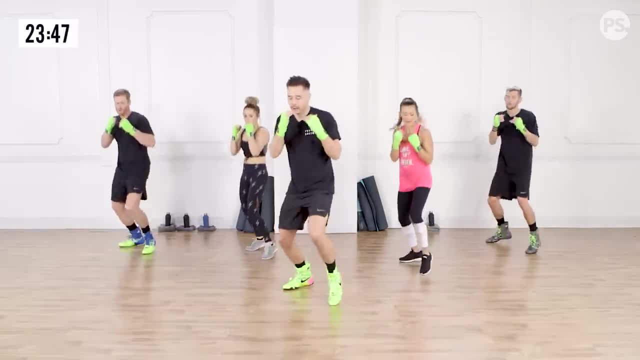 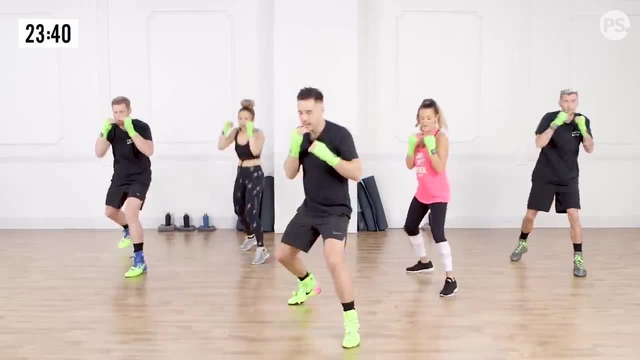 doing exactly the way that I'm doing it. Ready And go Boun boun, boun, boun And back. Okay, One more time And go Boun boun, boun, boun And back. Good, All right, Next portion guys. 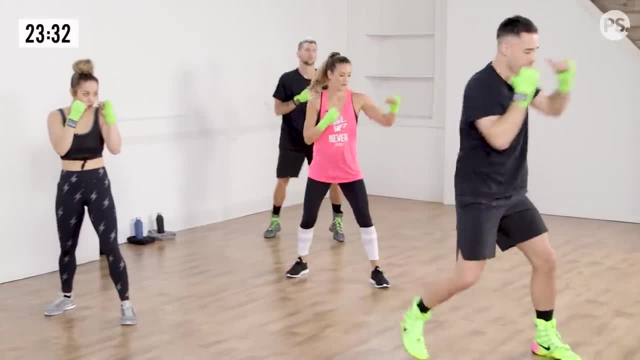 We're going to add a step back cross. So now I'm going to go one, two, One, two. I'm going to step backwards And I'm going to throw my cross. All right, So that's going to be almost our. 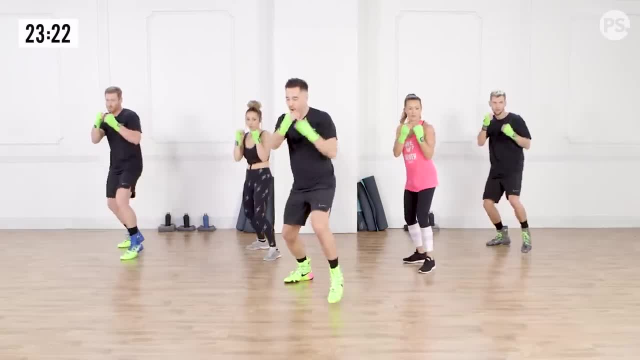 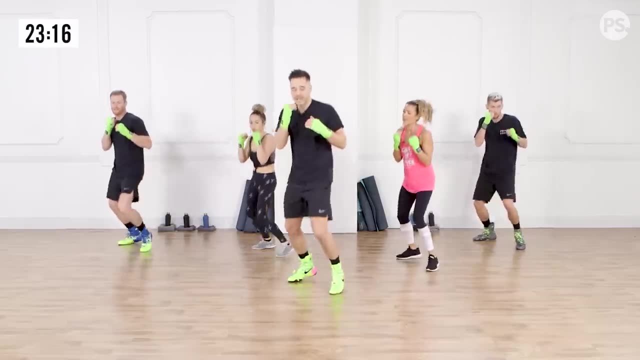 entire combo Ready From the bounce And go One, two, One, two, Step back, Two, Back to bouncing as soon as you're done, All right. So we keep that heart rate up Ready And go One, two, One, two. 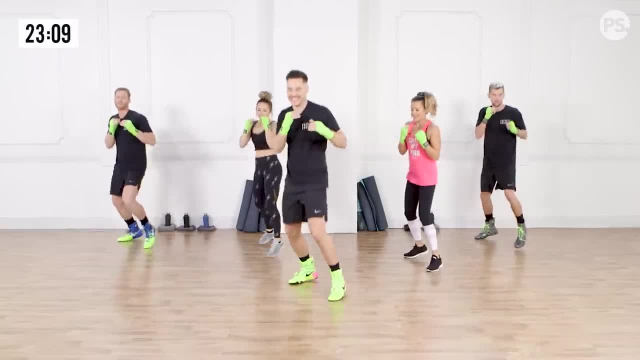 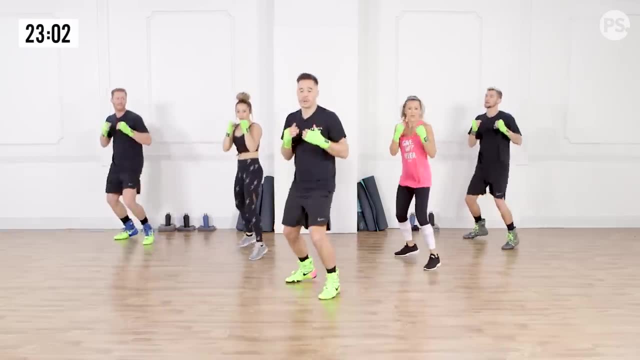 Step back Two. Good, Turning those hips is hard, you know, to remember everything, Yeah, So just keeping it at the forefront of your mind that goes a long way. So you don't have to do it perfect every time, but we just want to be aware and see where we can improve each time. 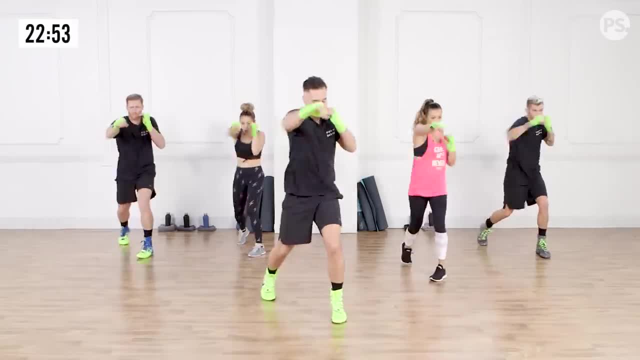 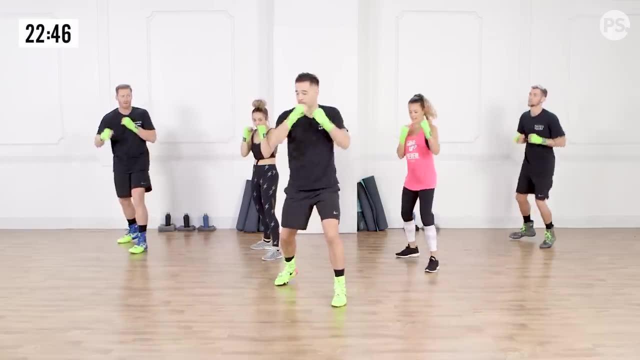 Ready And go One, two, One, two Back Down. Good, All right, Last portion of the combo of the day. All right, You're going to step back, cross, jab cross. So it's a one, two, One, two Step. 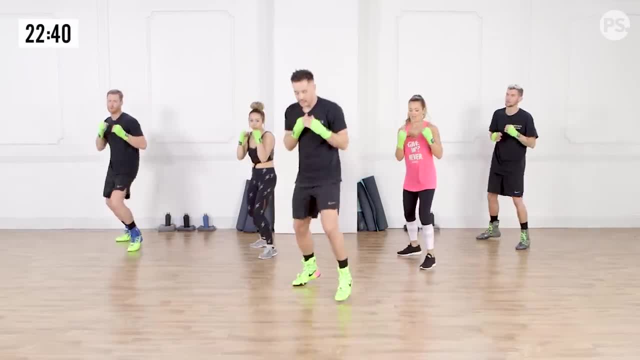 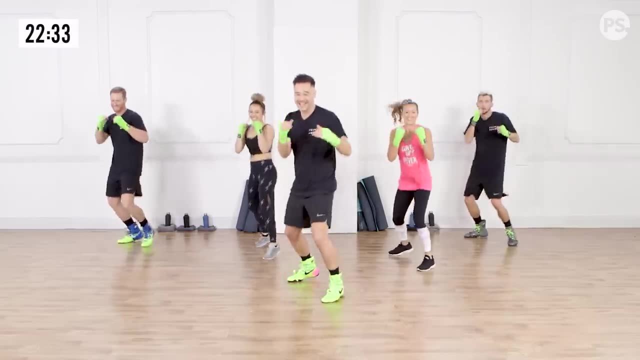 back Two, one, two. All right, So we're bouncing. If you guys need a simpler version, follow along with Waylon. This is the big daddy Ready And go One, two, One, two. Step back Two, one, two. 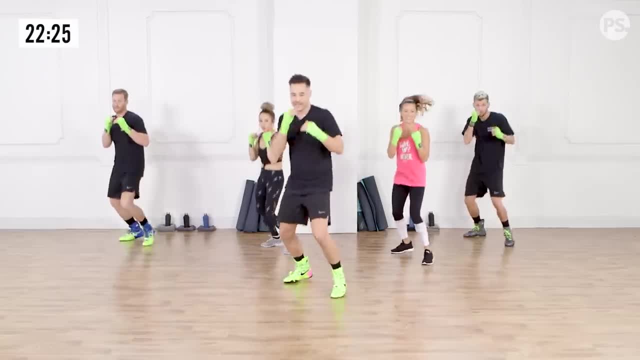 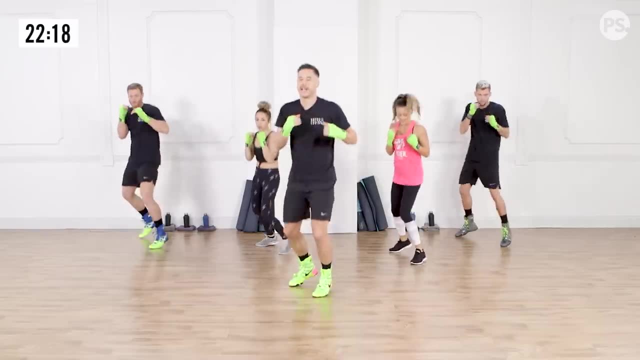 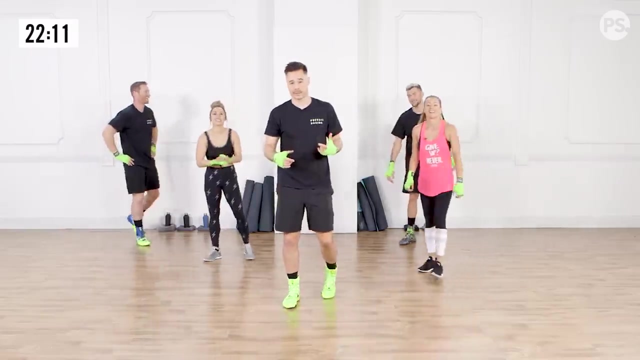 And bouncing. All right, Ready And go Back. Two, one, two Good And bouncing And break guys. All right, Nice work, Awesome, Nice work, guys. So that's our first boxing section. So now that we're warmed. 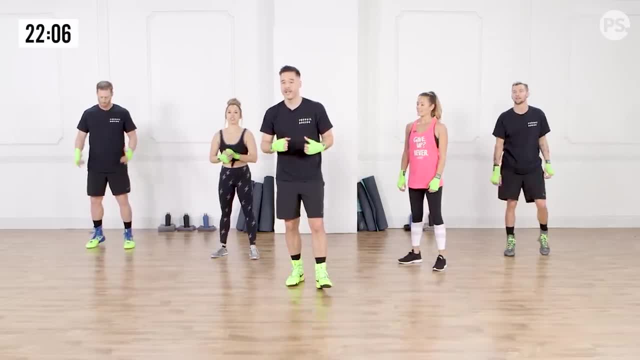 up. we got to do something a little bit to get the heart rate up All right. So we're going to go a little bit of a Tabata circuit. Tabata means 20 seconds of work, 10 seconds of recovery and we're. 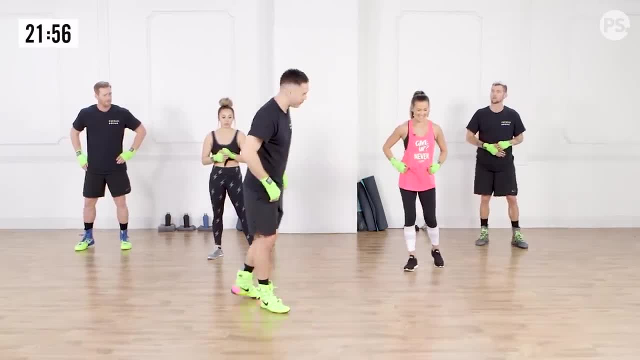 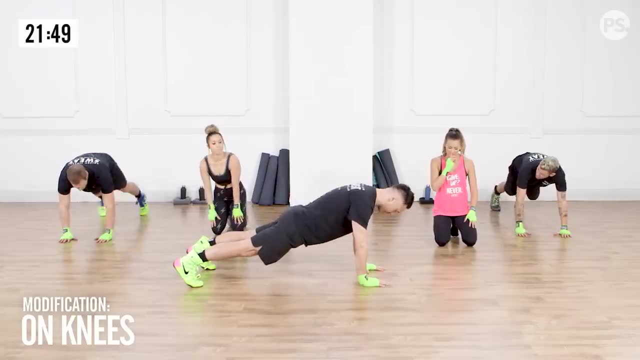 going to attack the upper body. Our first exercise, guys, we're going to be down in push-up position, All right, So we're starting off with shoulder taps from the push-up position, So we want to be here back flat. Okay, Stabilizing through the core, tapping shoulder to shoulder. 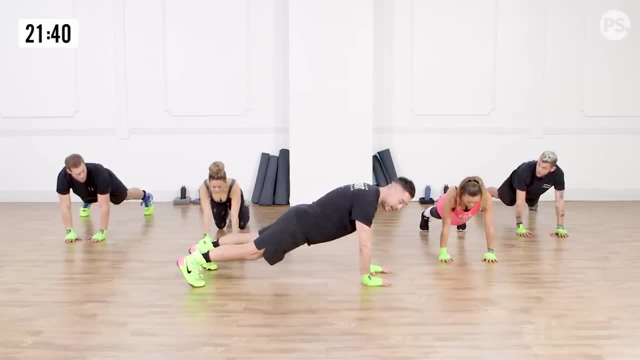 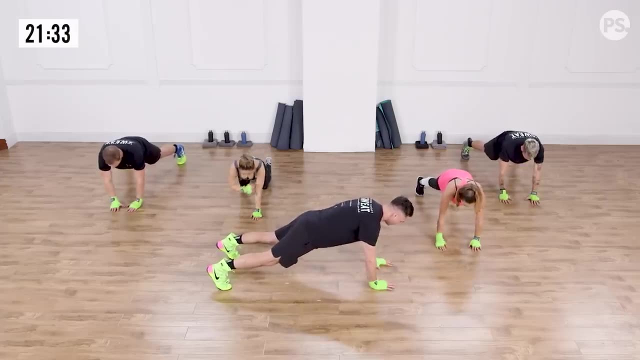 All right, We're going to go for 20 seconds And go, Make sure that again we're stabilizing through the core, trying not to let the hips move. All right, That's the hard part. Feet wider is easier, right. 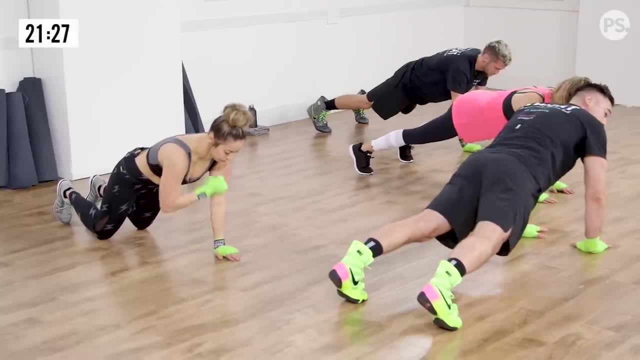 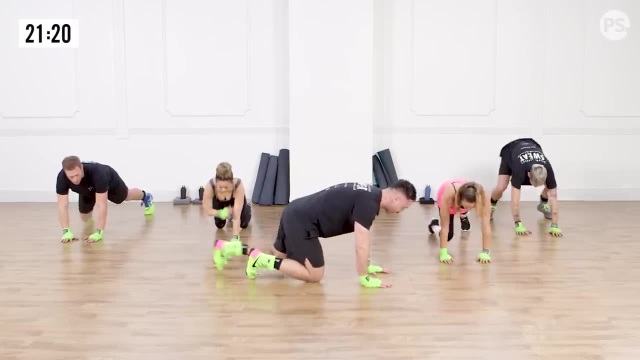 Feet wider is easier, or you can even do these on your knees, All right. We got about five more seconds. You guys are doing awesome, Very nice, And break All right Way to earn that break, All right. So in order to earn that break, we really got to sprint for those 20 seconds and then we 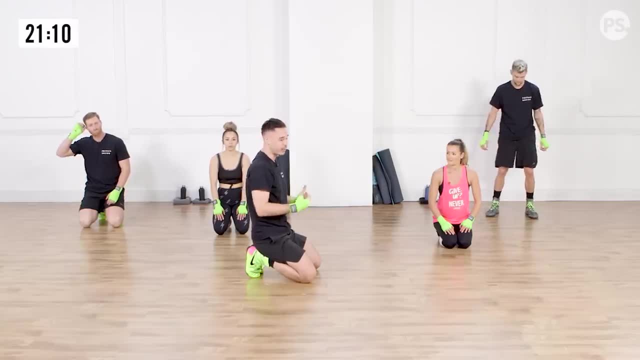 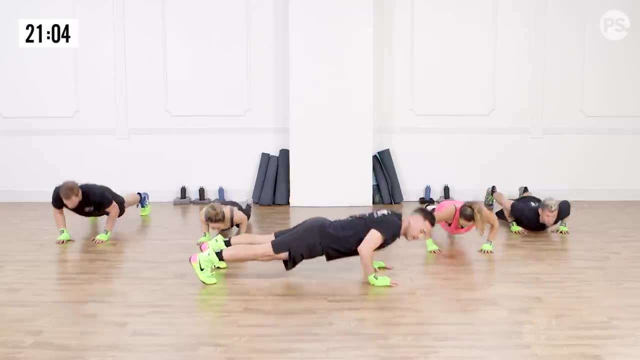 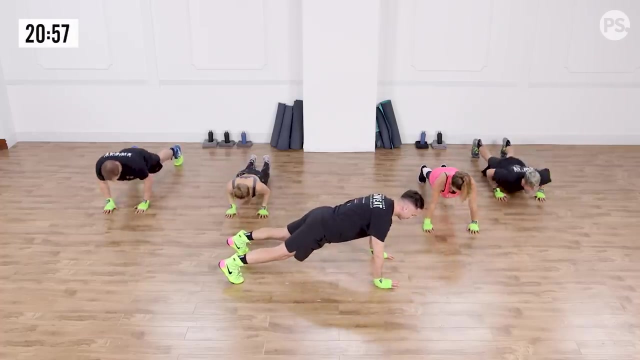 have 10 seconds to recover, So a lot of boxing is going to be sprint intervals. All right, Yeah. Next exercise we're going to go push-ups. All right, 20 seconds Ready And go. So when you're doing the push-ups, I want you to imagine that you're pushing the earth down and exploding up. 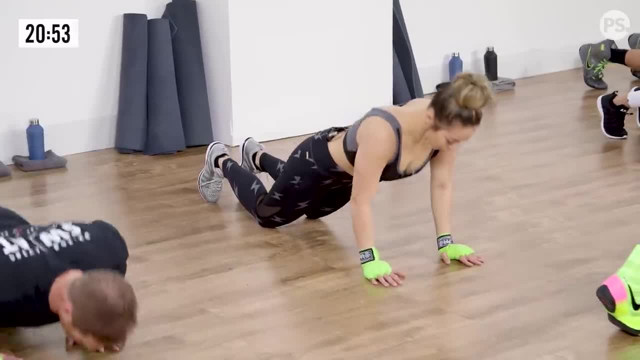 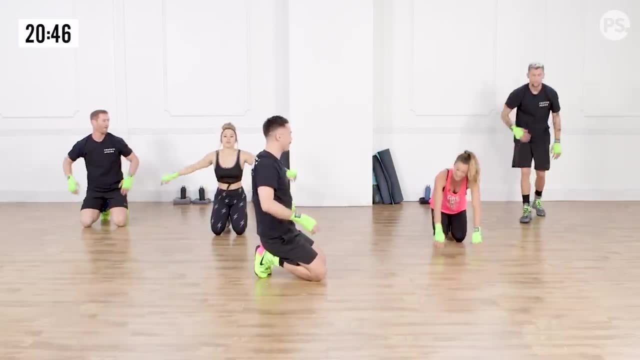 All right, Good Back flat core engaged. Oh yeah, Woo Good And break. All right, pump, Shake out those arms. We earned this 10-second break. All right, This next exercise is going to be push-up. 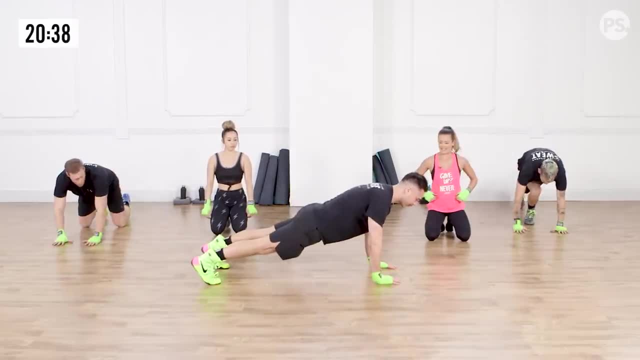 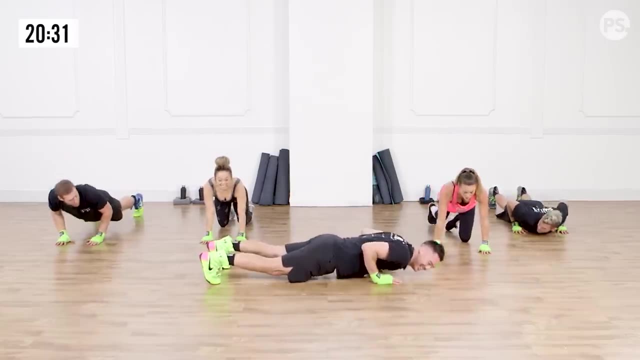 pulses. So we're going to stay low to the ground. All right, Same thing. Back is flat core engaged. We're staying low, bouncing Lovely. All right, Let's do it, Let's get it. Wait, wait, Oh, we're already starting. Okay, Sorry. 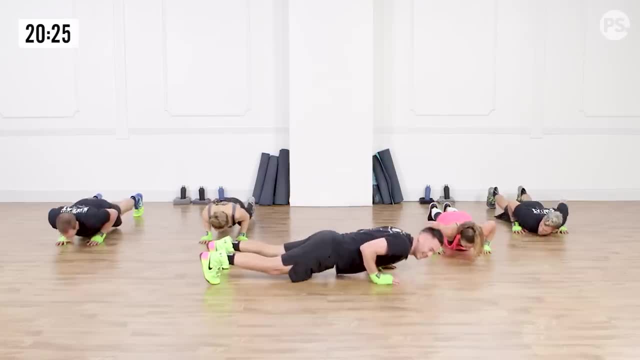 The clock does not wait for anyone. No, Sometimes you got to chase the greatness down, you know, Oh my gosh. So, All right, Staying nice and low. Three, two and one, All right, We're going to sit back, shake it out. We're going to run through that one more time, All right. 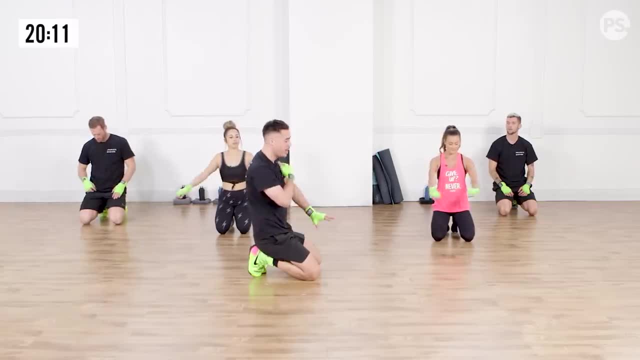 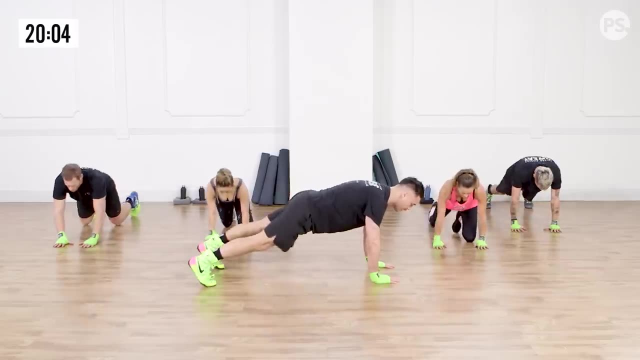 So we're doing three minutes total work. All right, We're starting off Shoulder taps, Remember, stabilize through the core. Try to keep your hips parallel to the ground. We're starting in three, two and one. Good, Does it matter how fast I'm tapping? 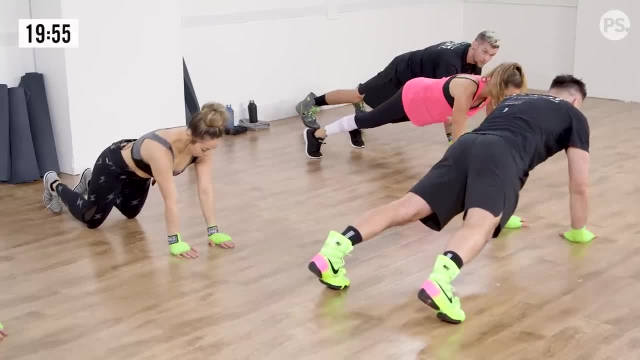 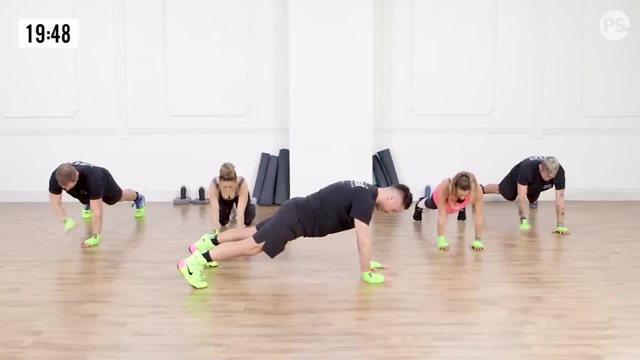 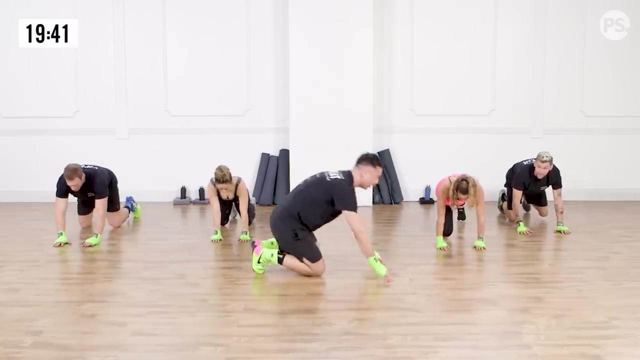 No, I think the most important thing is where you're getting your stability from Right. So you should feel it in your core. Feels great. Nice work guys. Abs on fire, Abs and shoulders Good And break. All right, We're going push-ups. next Ten-second breather: Shake it out. 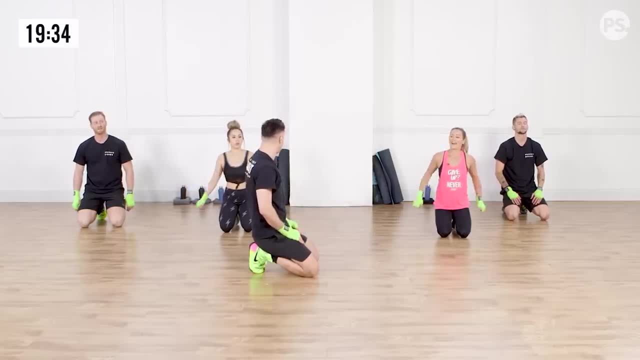 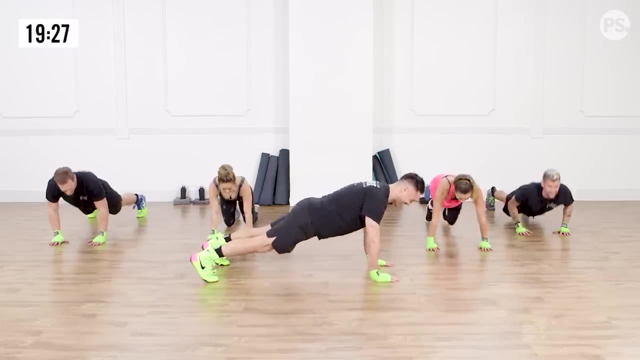 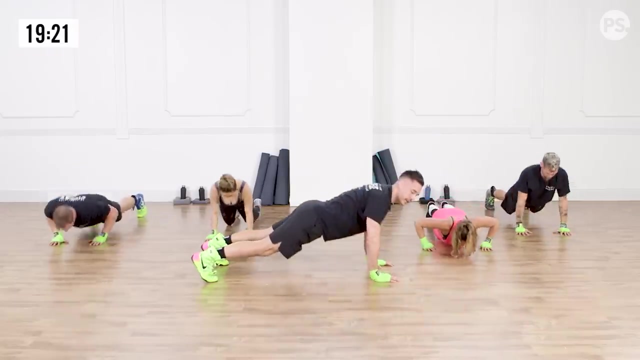 We're really attacking the upper body in this sequence. Yeah, I feel that Hopefully everyone's feeling that It feels attacked. All right, Push-ups, Here we go. Still love you, Still love you, Full range of motion, And again you can do these from your knees, But, most importantly, try to stay moving. 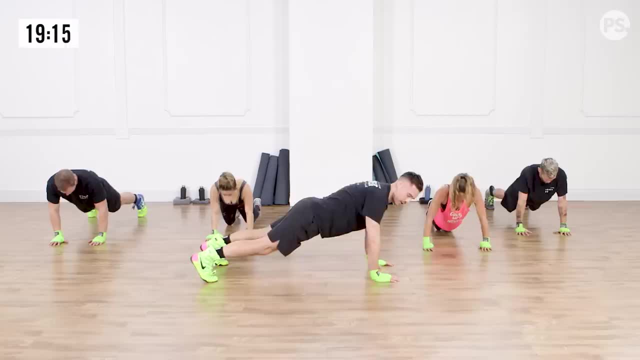 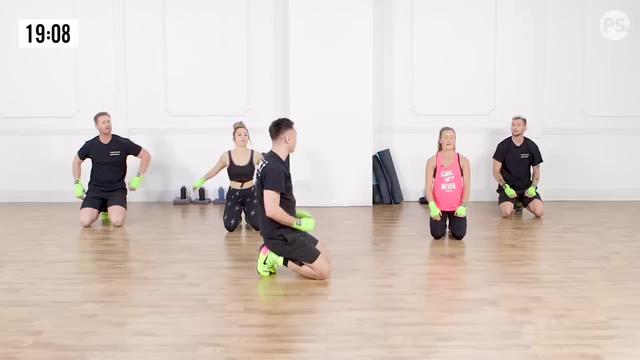 Exhale on the way up And break guys Ten-second breather. Doing great. We got one 20-second sprint left. That's going to be those push-up pulses. Let's get it. Let's do it coach. 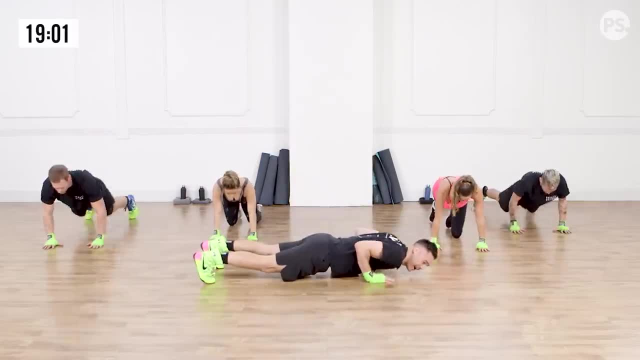 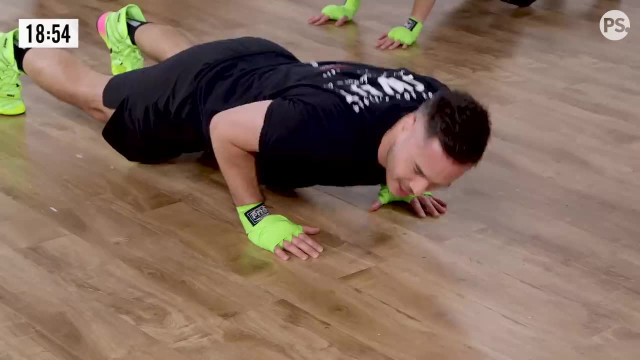 50 of them. Feel strong. Here we go, Here we go And pulse it out. Try to keep that back flat. Last one for the muscle. You might start to feel a little something in your arms. That means you're doing it right. 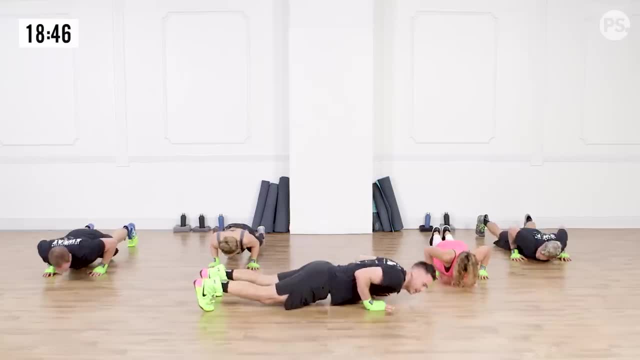 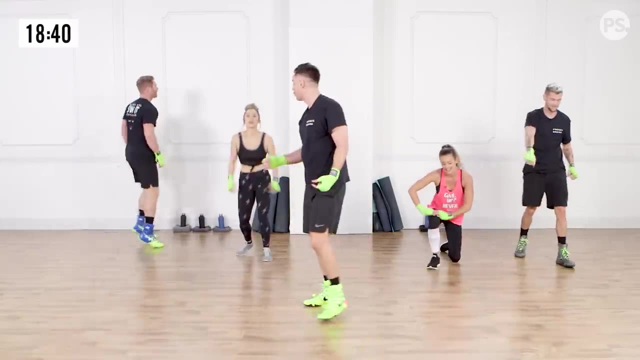 Good, Five more seconds, Three, two and one. Nice work, guys. Excellent. All right, Shake it out. You guys did awesome. So for our second portion, I'm going to actually bring up Coach Rob, All right. 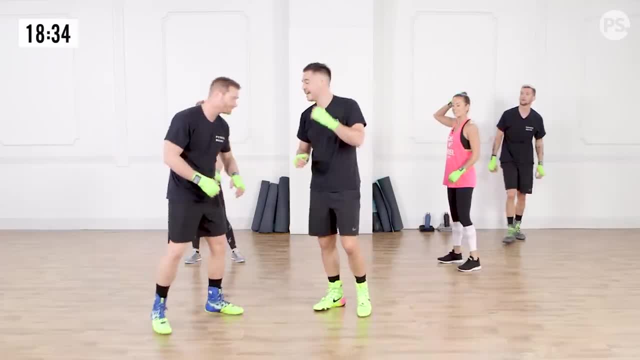 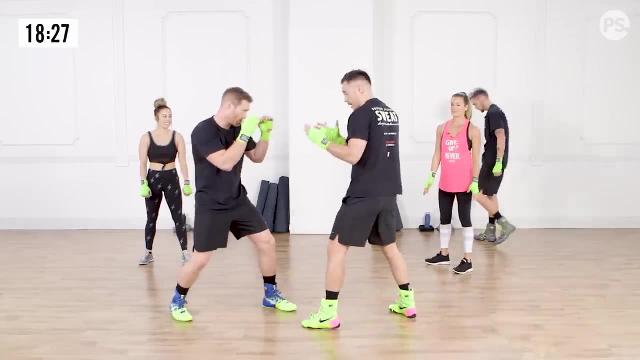 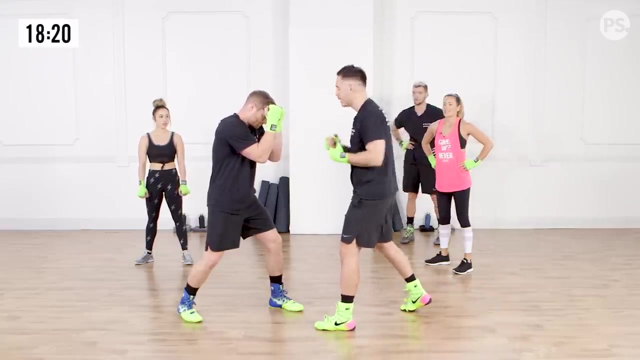 So I brought Coach Rob with me from Prevail. We're going to be focusing this next portion on working on our hooks and slips. So the hook: if we're actually sparring each other. if my opponent decides to put his guards up close like this so I can't hit him with a jab cross, which is what we just learned- I'm going to go around his guard and hook from the side. 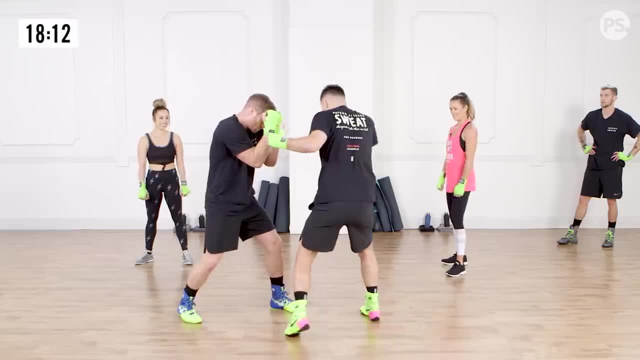 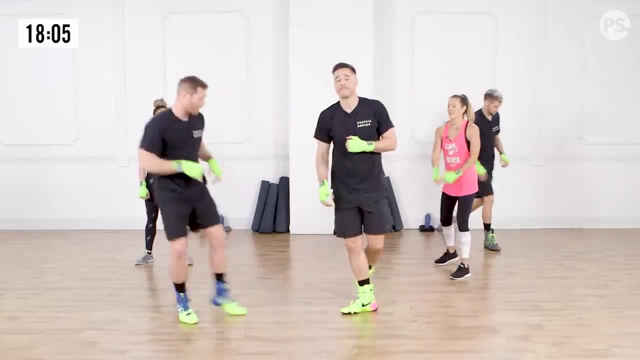 All right. So you'll notice that when I throw my hook, I'm pivoting and rotating my hip and my foot with the punch Boom and bang. All right, Thank you, Coach. Yeah, Rob, So the power comes when we use our entire body. 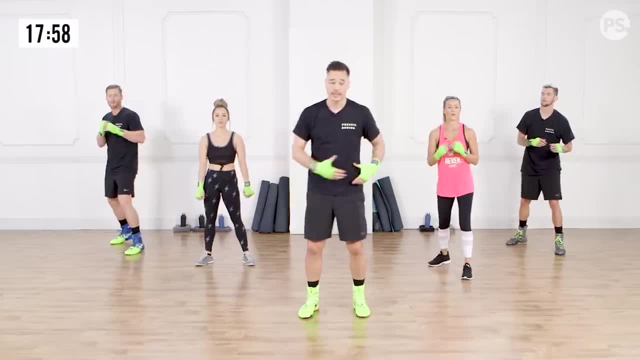 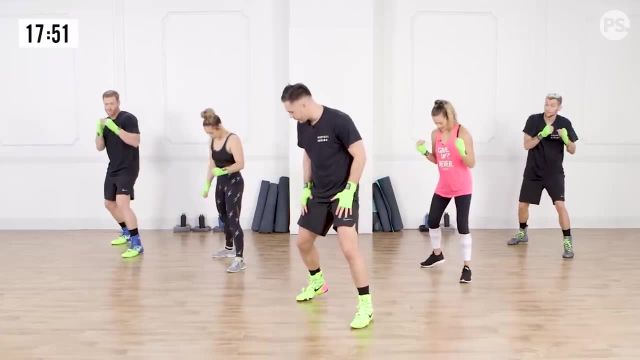 It's not about big arms, It's not about a big chest. It's about using your legs, your core, your back and working in unison. All right, So we're going to start off nice and easy Again. good boxing stance. 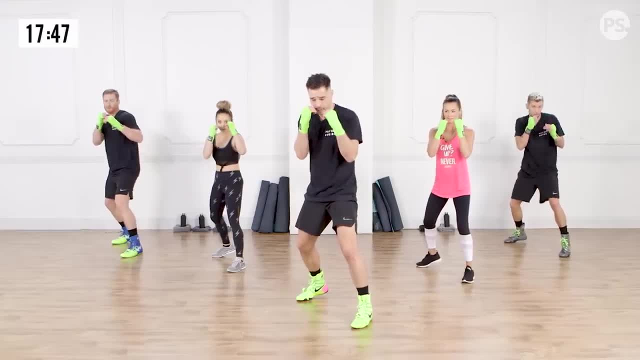 My back heel off the ground. Hands are up nice and high. From here, what we're going to do is we're going to pivot our back foot, rotating our hips and shoulders, And what we're doing is we're setting ourselves up. 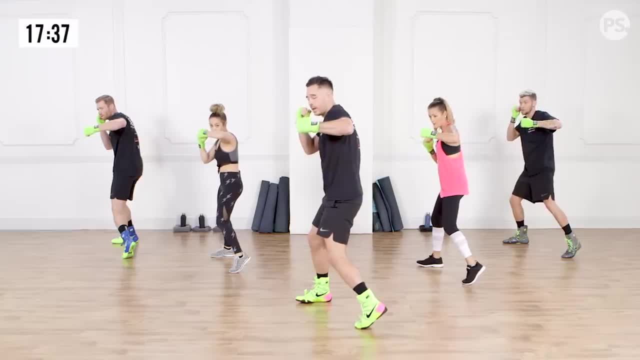 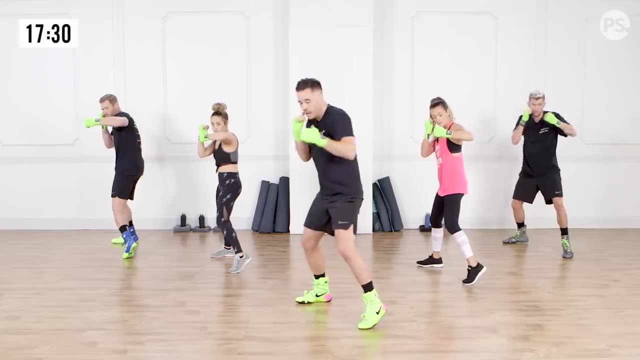 So that we can generate power in our left hook. Now, when I'm throwing my hook, elbows bent at 90 degrees, Thumb is facing up Back. hand up nice and high. From here we're going to reset, All right, So I want everybody in the bounce. 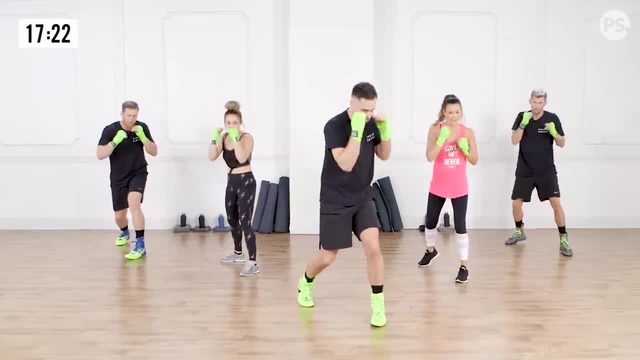 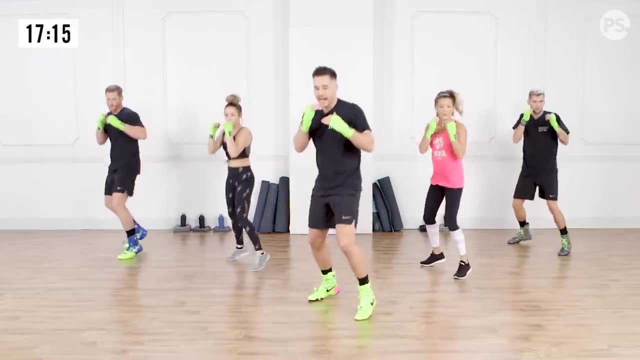 Okay, When I say go, you're going to plant your feet, You're going to rotate your hips and throw that left hook, Then back to the bounce. so I know that we're ready. All right, Ready And go, Plant the feet. 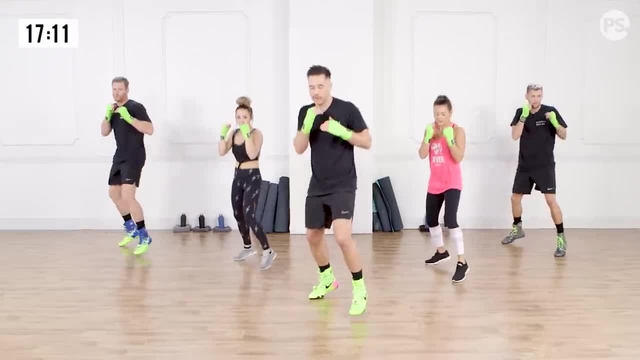 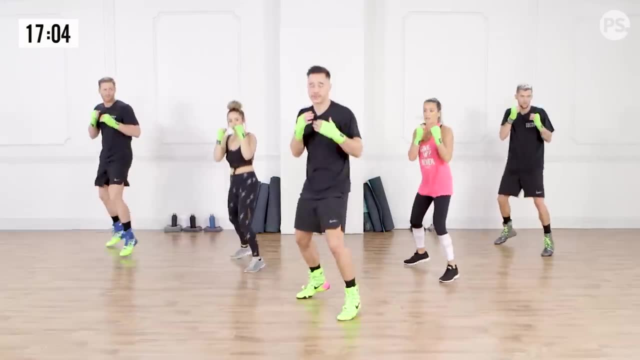 Hop Bang Back to the bounce. Good, And go Boom And back to the bounce. And the reason I'm having you guys do it to my command is so that you have to stay ready the entire time. So you have to be present and you have to be focused. 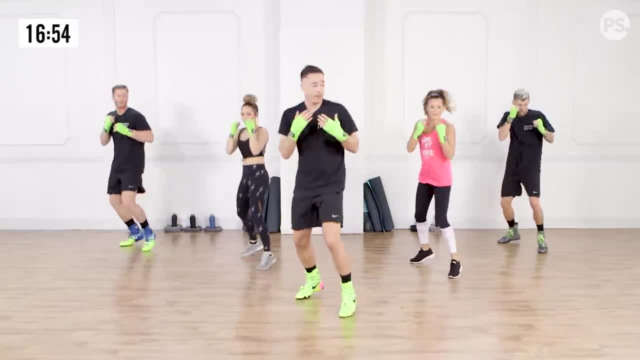 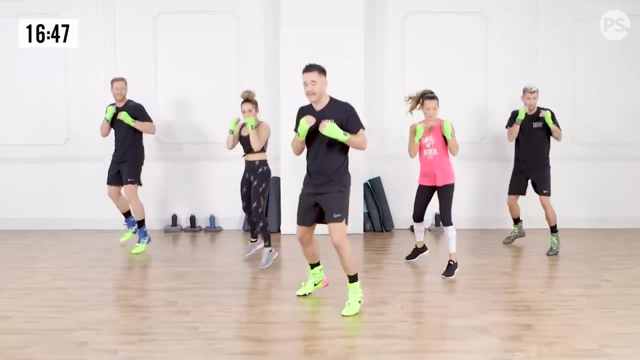 Just like you would have to be if you were boxing Right. Yeah, So my opponent wouldn't stand there for me to let them hit them Right. That's true. Yeah, I'm not waiting for you. So when I see the opportunity, I have a split second to react. 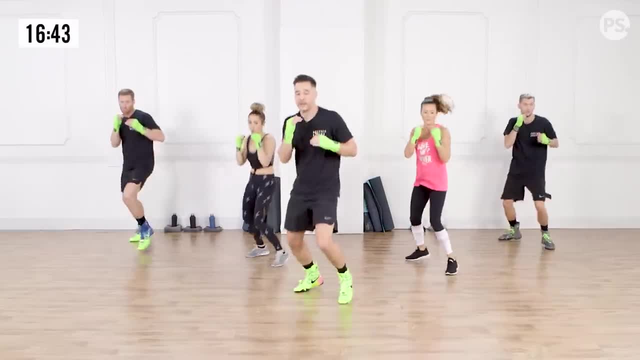 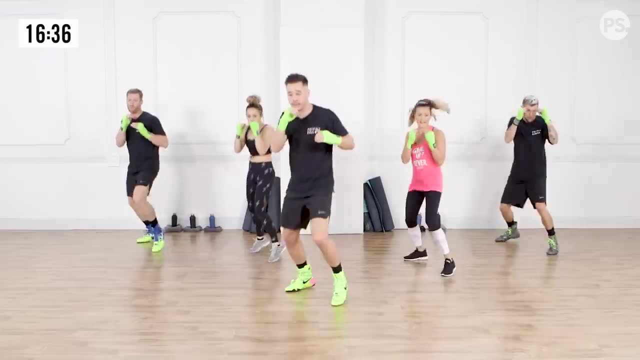 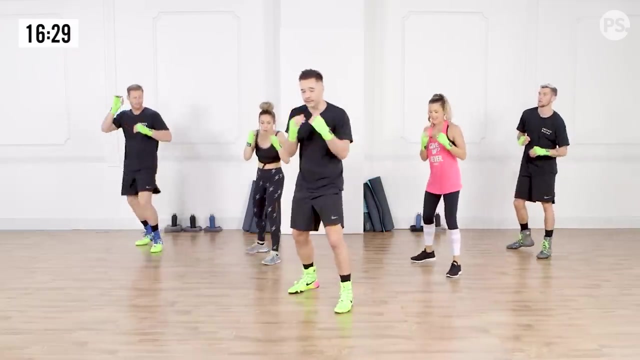 And that's what we're doing here. Go Boom And right back Ready. Go Hop, Hop Right back. And go Hop, Hop Right back, Nice guys. And one more: Go Hop Good. 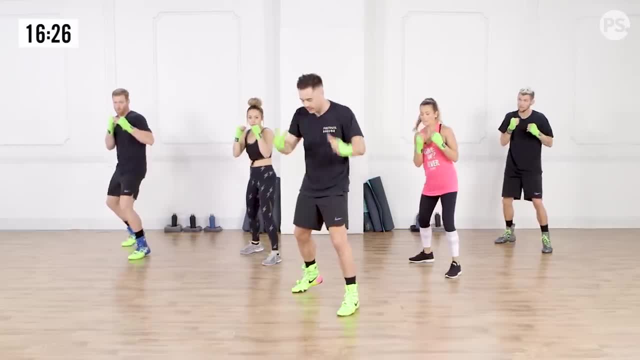 So now we're going to work the inverse. All right, That was our left hook, Now we're going to work the right hook. So from here we're going to bounce. When I say: go, you plant the feet, We're going to dip down. 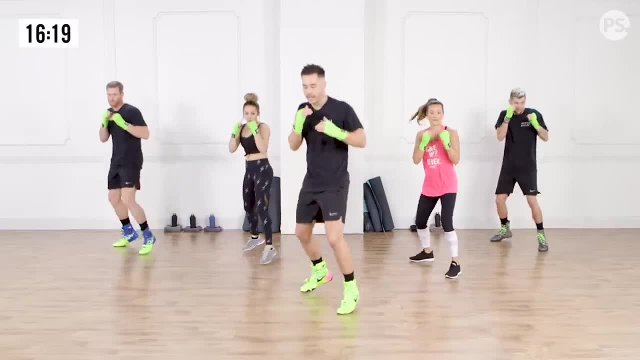 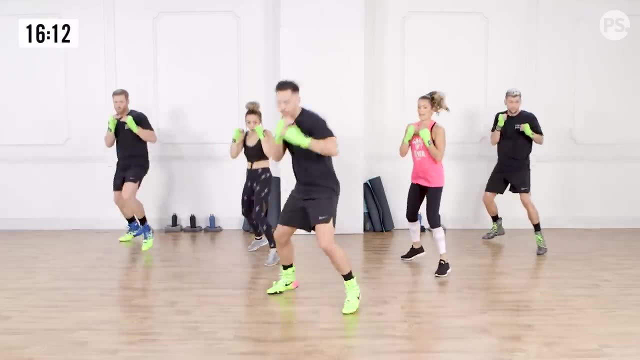 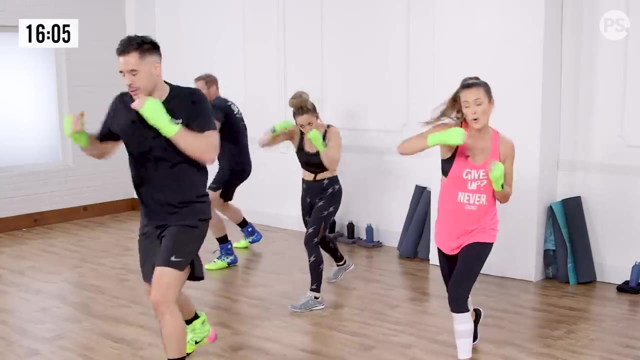 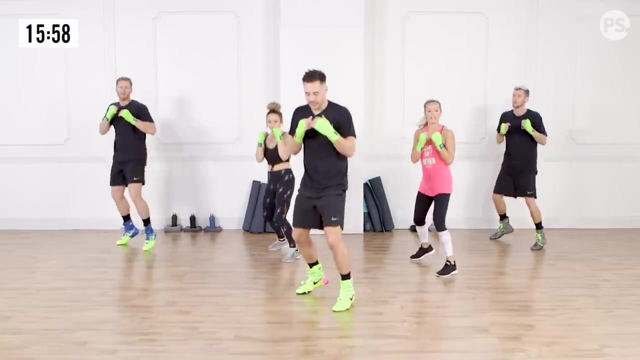 Right hook Right back to the bounce. All right From here. And go Hop, Bang Good. And go Bang, Go, Hop, Bang Good. Staying light on those feet, Go Go Good. This time we're going to add a double slip to it. 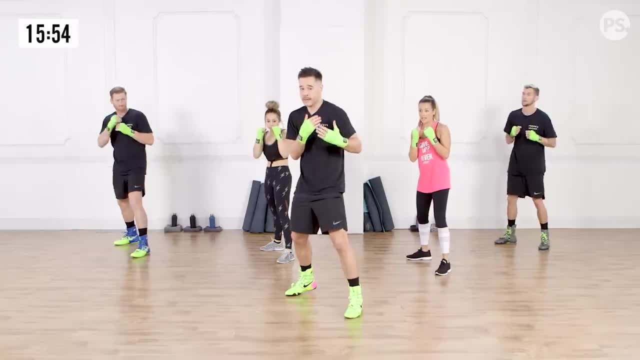 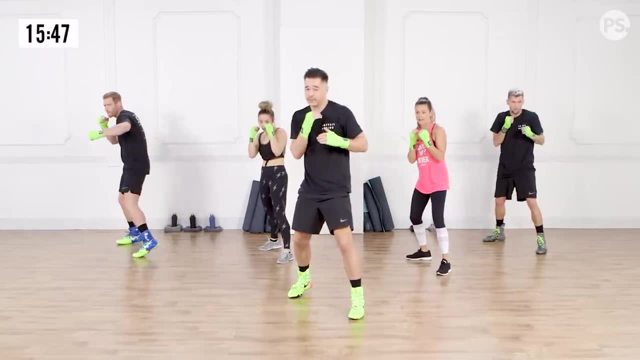 So slip is basically a head movement that makes my opponent miss when they're attacking me. All right, So if they throw their jab, I'm going to move my head out of the way Left And then to the right for the cross. 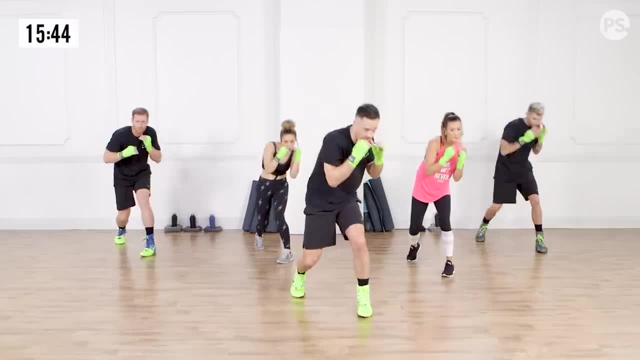 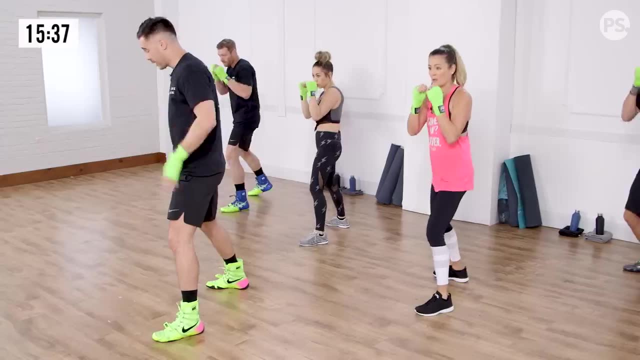 So we're going to do two movements: We're going to go to our right and then to our left. I'm pivoting my back foot so I can stay nice and balanced, And I'm keeping my hands up high. All right, So we're here. 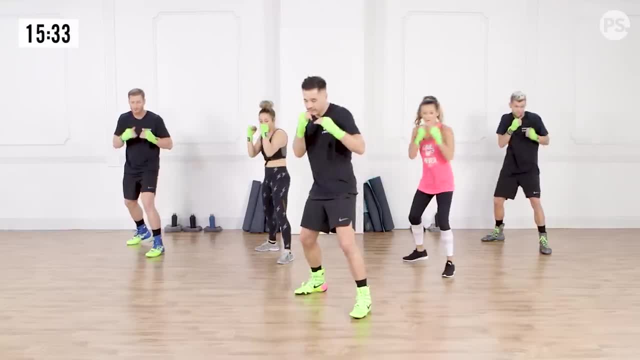 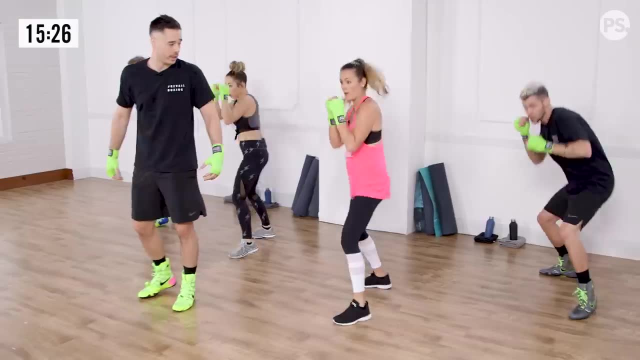 Plant your feet for this one. And when I say, go to the right, to the left, Reset All right, Ready And go Good, Keep those hands up, nice and high And go Good, Ready, Go Hop. 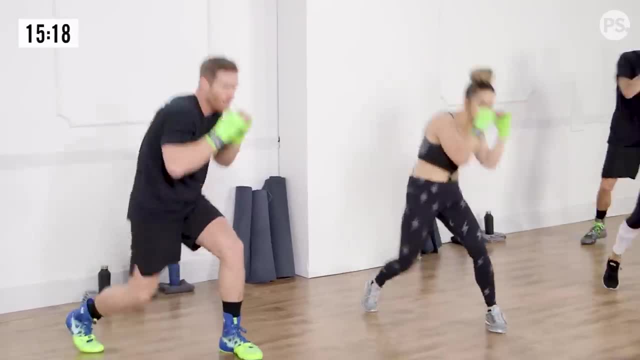 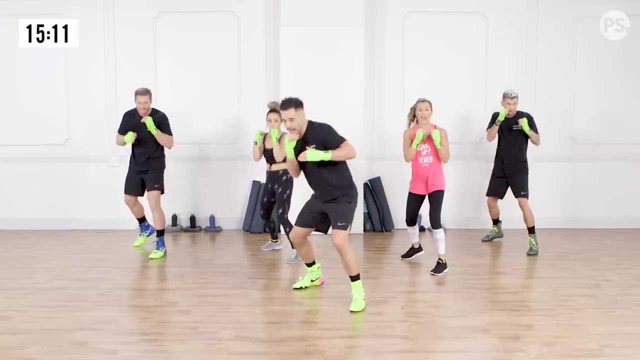 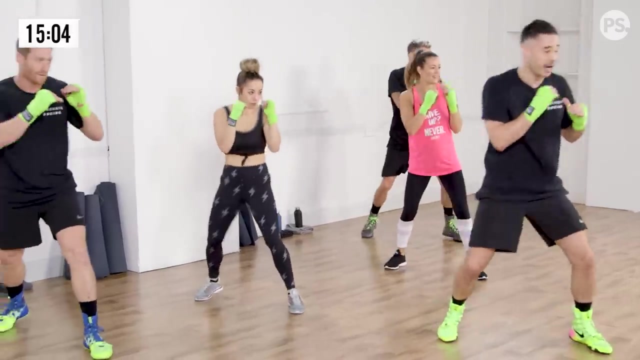 Hop, Very nice, And go, Bang, Bang, Go Go. We're going to go to the right and left first, OK, So right, then left. Ready, Go Hop, Hop, Good, Go, Hop Hop. 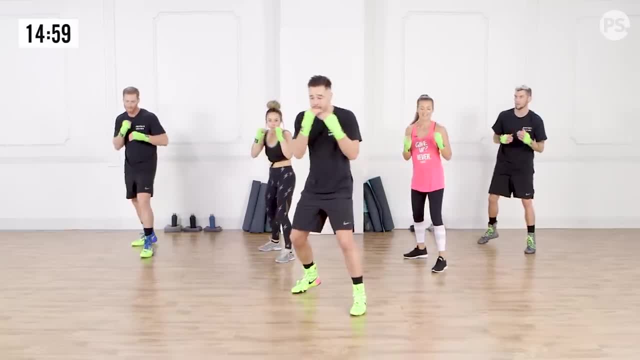 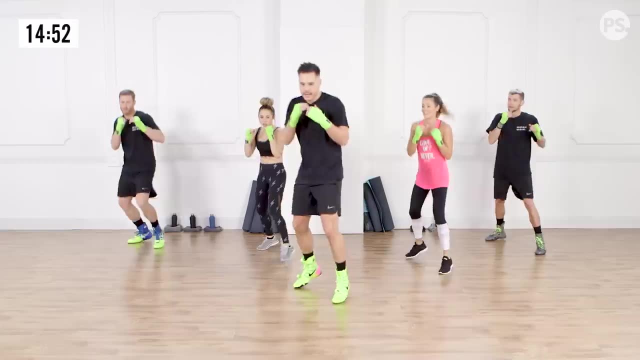 Good, Go, Hop, Hop, Nice, All right guys. So let's add. Let's add to that: You guys are doing awesome, So we're just going to keep building it up, All right. So here we're going to slip. 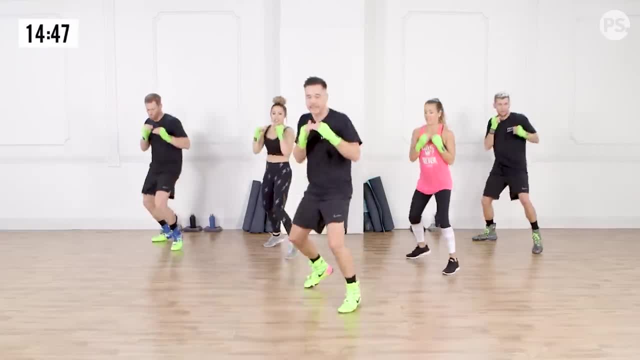 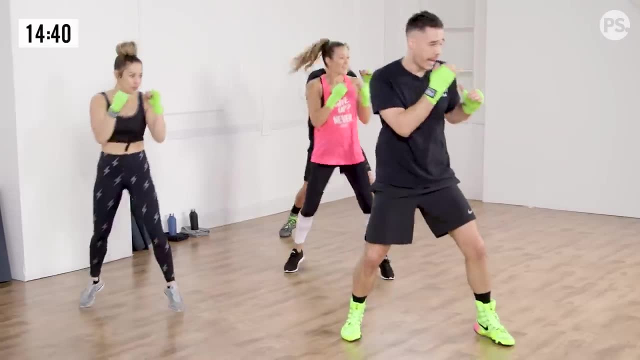 Slip Slip big beats. Slip slip Bum bang Back to bouncing. so I know you're ready, Ready, Go, Hop, Hop, Bang, Bang. Good And go, Chhh, chhh, Boom. 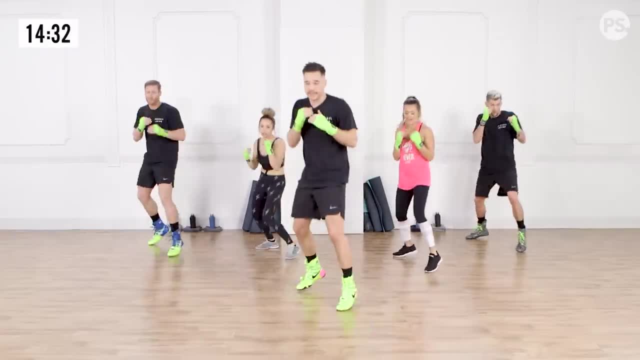 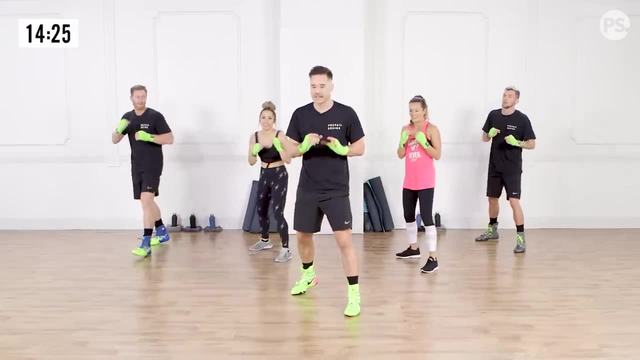 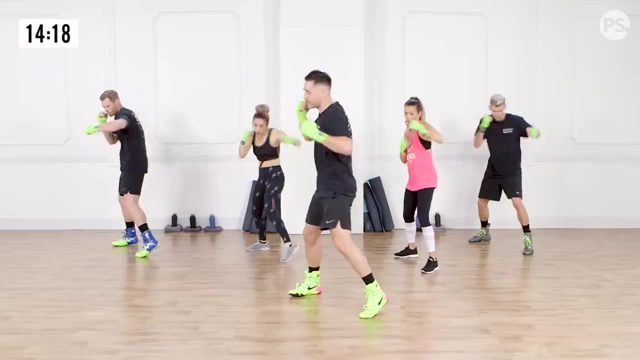 Boom, Good, Go, Hop, Hop, Bang Bang Nice And go Hop, Hop, Boom, Boom. Good guys, We're going to go 30 seconds. I'm going to try and improve it 1% every time, okay. 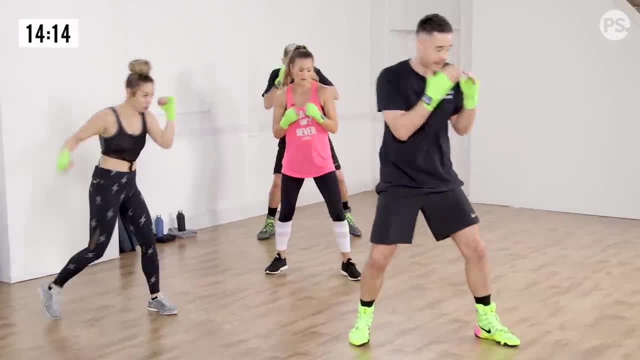 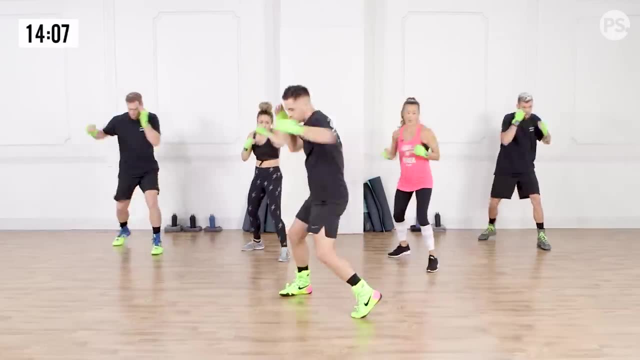 Whether it's just balance, speed, power, keeping the hand up, something, All right, Go at your own pace. Hop, boom, hop. You'll notice I'm using my entire body every time I punch. Hop, hop, hop. 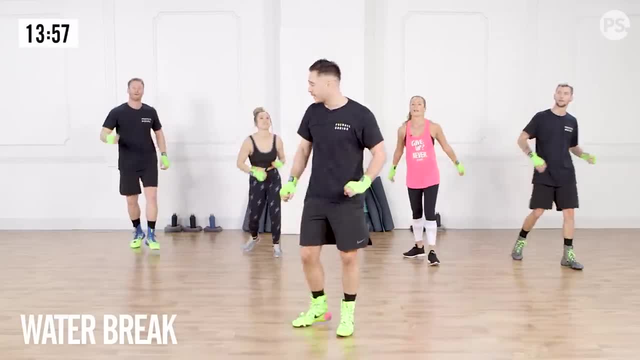 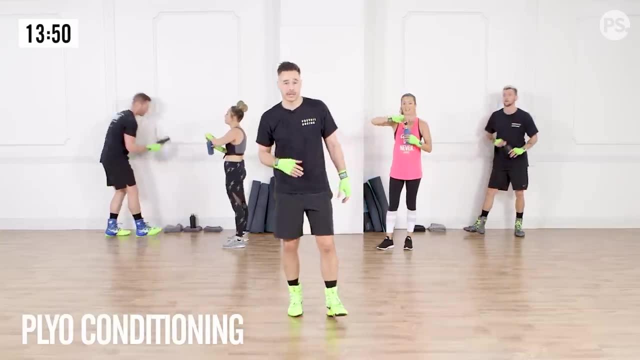 Good And break guys. Nice work. We're going to take a 30-second break right there. You guys are crushing it. You guys are crushing it. All right, we're going to go into a three-minute plyometric conditioning. 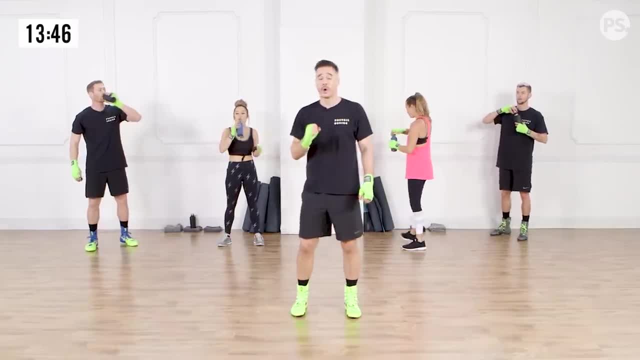 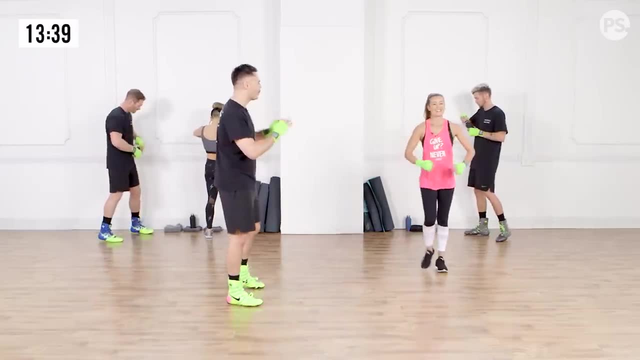 All right For the first minute. guys, we're going to go squat thrust. The goal, the challenge, is to hit 20 squat thrusts in one minute. Anna, would you mind demonstrating that? perfect squat thrust. There we go, Anna. 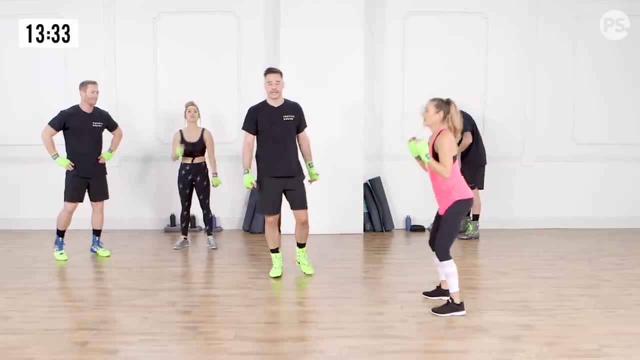 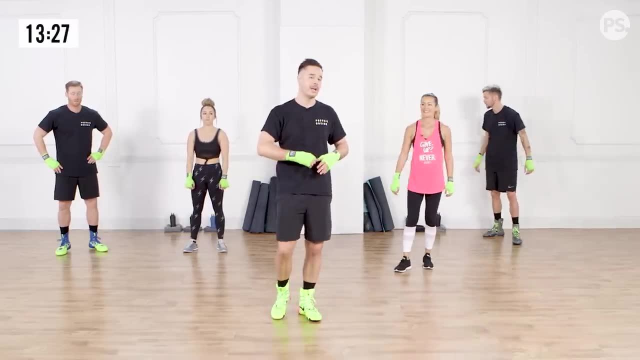 All right, Here Down in push-up position, bring the feet in jumping up at the top. So this is a full-body plyometric movement which is meant to be explosive and helping you develop your cardio And your ability to kind of hop off the line and throw a powerful punch as well. 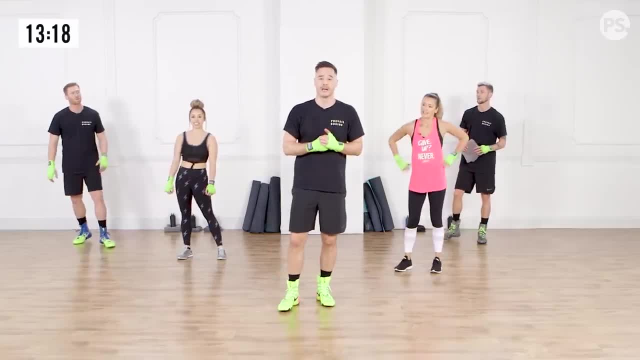 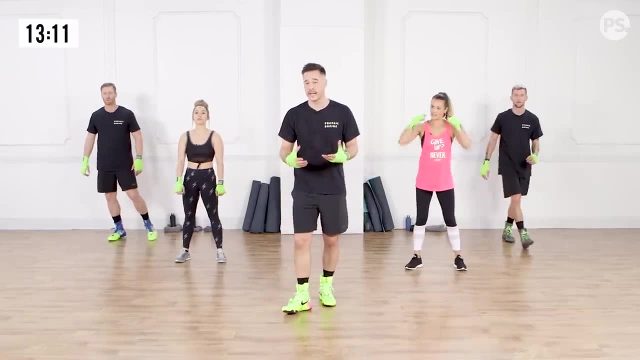 All right. So it's great for boxing. It's super challenging, but we love taking on challenges, All right? Yes, So we're going to go in 10 seconds. We've got one minute to do as many as we can. 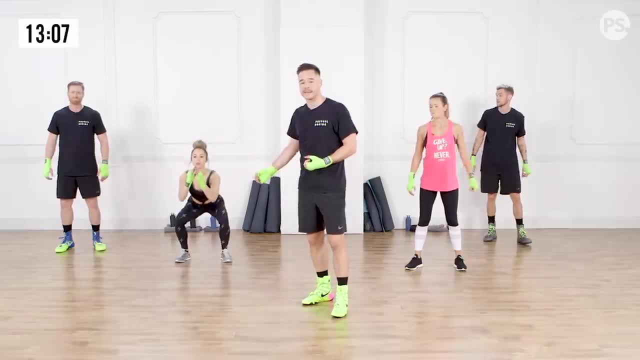 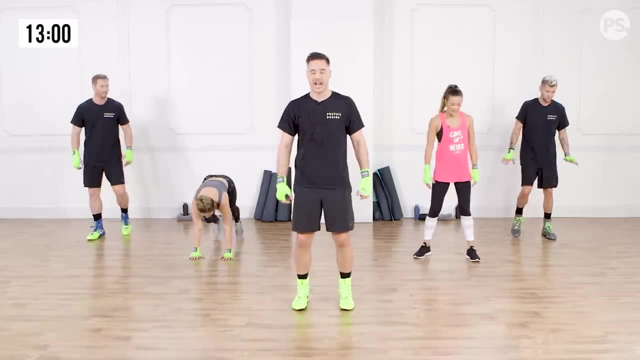 A modification. you can start off simple with squats. If that ends up being a little bit too easy, you can do a walk back and then just walk right back up. All right, We've got one minute. 20 is the challenge. 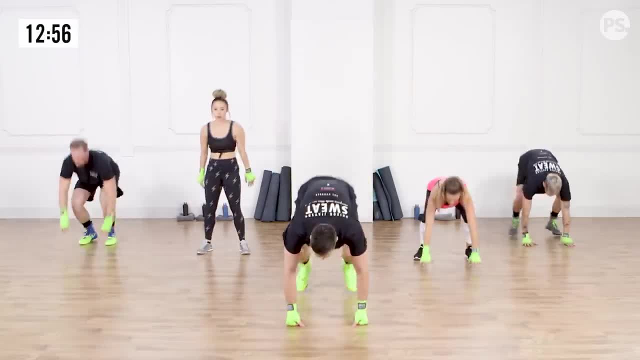 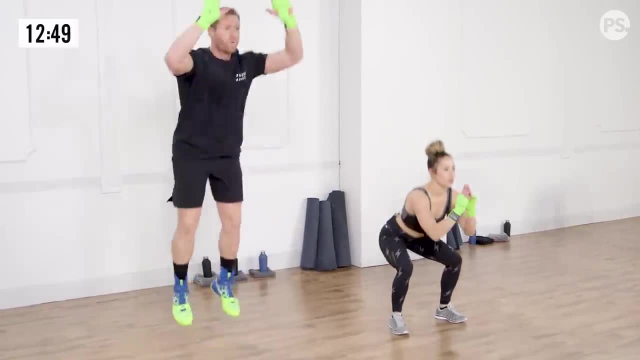 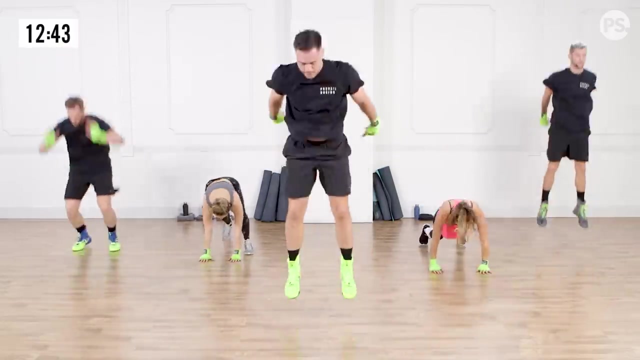 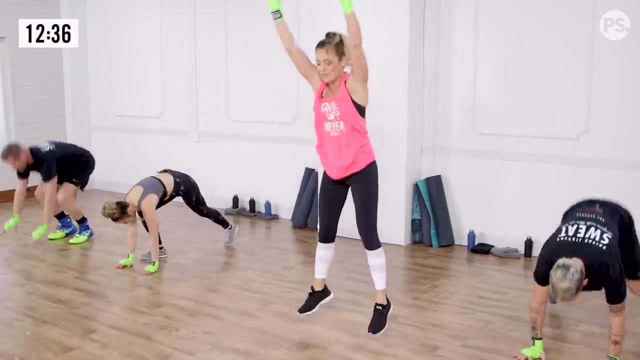 And go. Make sure that When you guys land, you land nice and light. All right, Woo Woo, All right. Oh yeah, We're getting ready for the ring right here. Let's go. Let's go, baby. 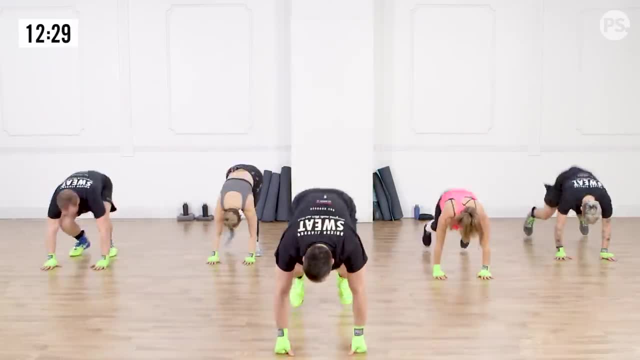 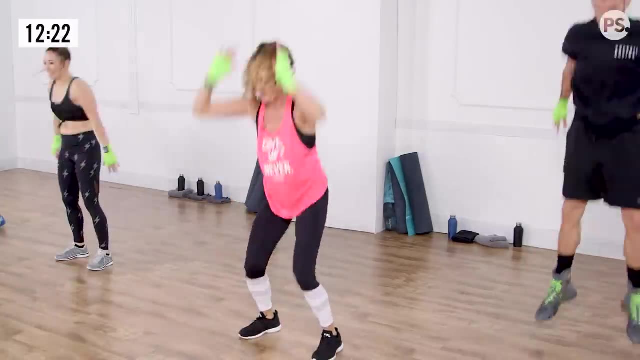 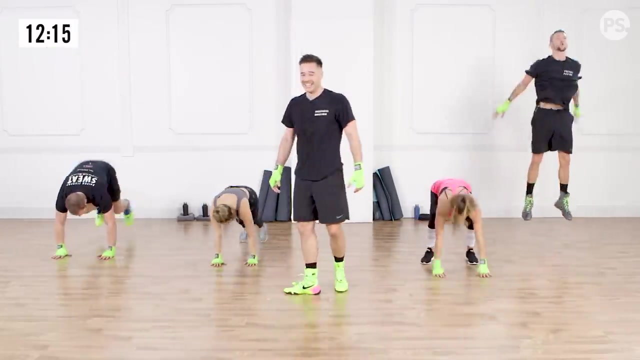 This is the easy work right here. I know I'm liking those hooks right now. It's better than me. That's my 20 right there. I don't know about you guys, I'm afraid. Okay And break guys. 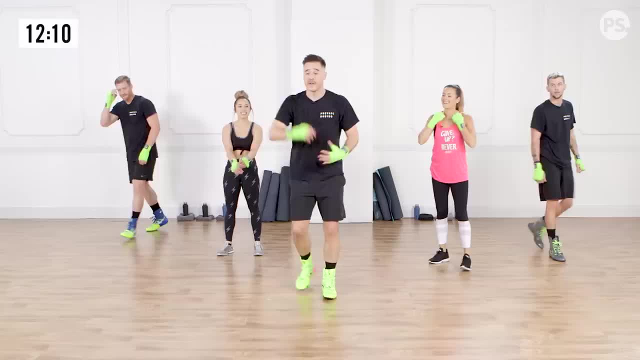 Woo, All right, We're going to go straight into minute number two. The challenge is 50 jumping jacks. Let's get it. And for We're going all the way up on these. All the way up, All the way up. 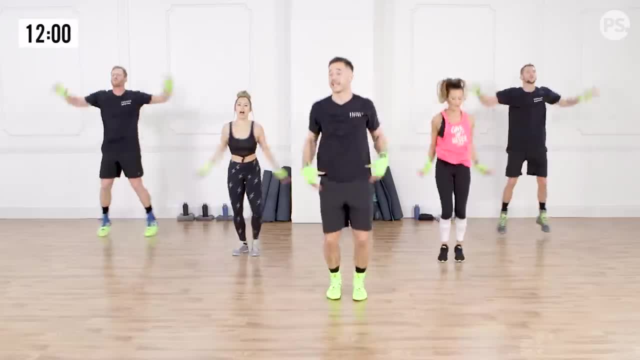 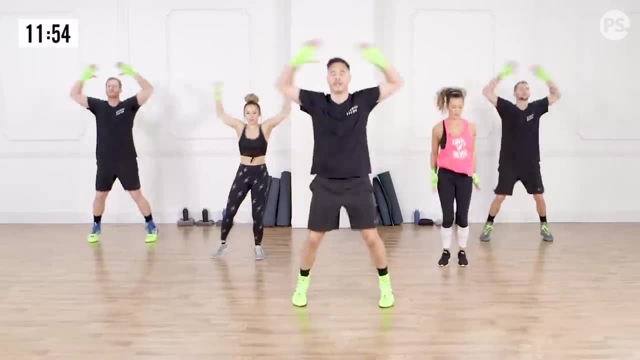 All the way down. Everything we do 100%. Again, if you guys need a modification at home, follow Leilani Right there with the step jacks. Now it's important to note when you guys are doing these. we want to keep the heels off the ground so we stay on the balls of the feet. 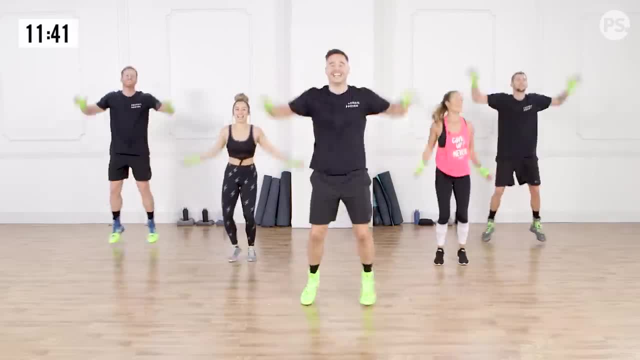 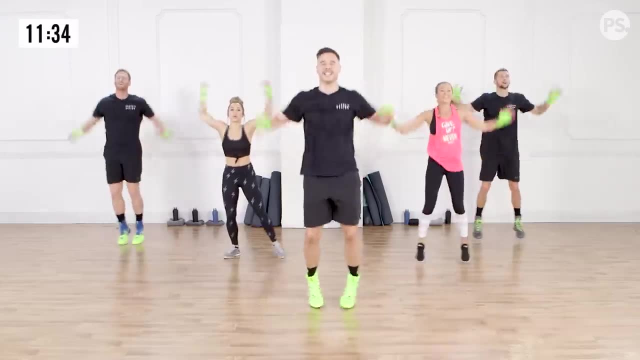 All right, Is anybody counting Guys? come on 36.. Oh wait, I was up. All right, You're going faster than me. You're good. Heels in my arms. Woo, There we go, All right. 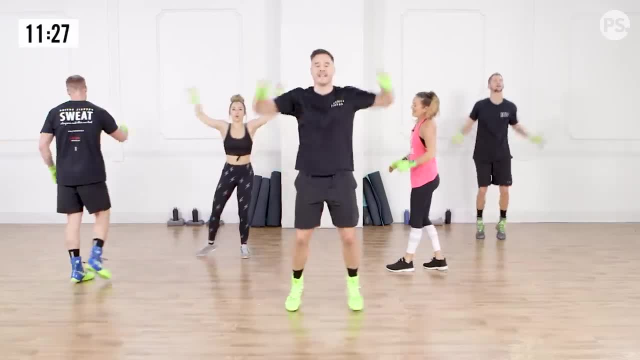 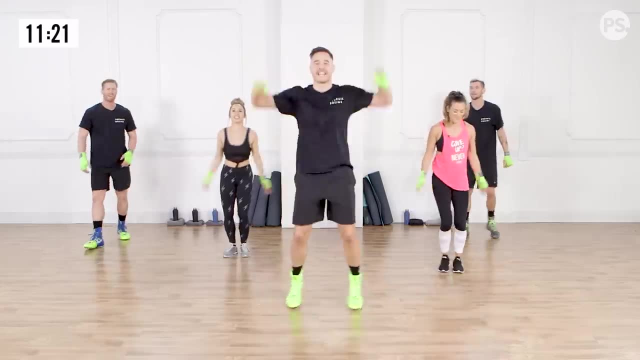 I'm finished talking about you guys. 10 seconds left. Let's get it. Let's get it. I like the countdown. Oh yeah, Five more seconds. I'm just going to go the whole time because I didn't count. 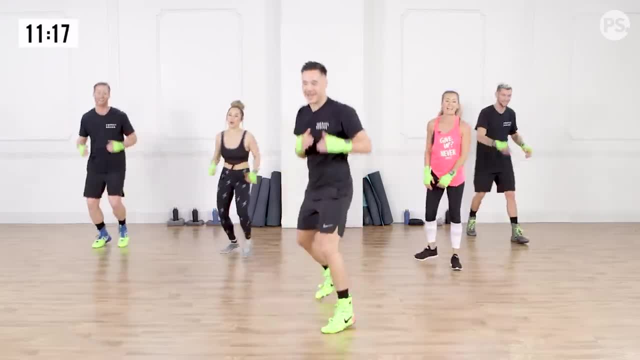 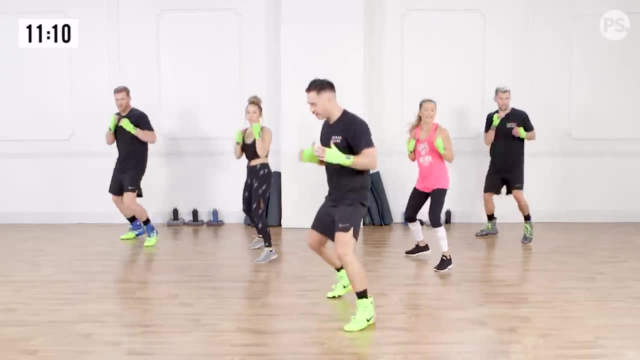 Oh yeah, Good, Good, Let's do it. Make us feel bad. back here, Milan. Let's go From here. guys, we're going to go 50 reps Forward and back Again. we actually want to cover distance as we're hopping. 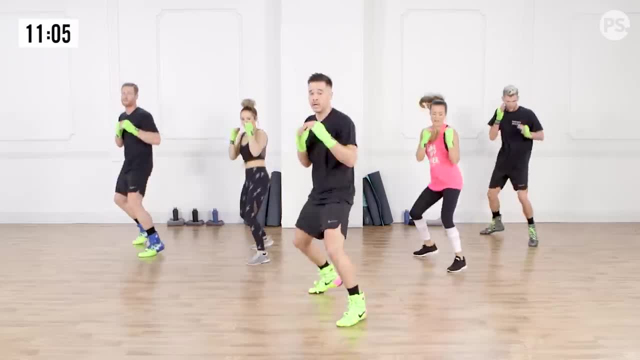 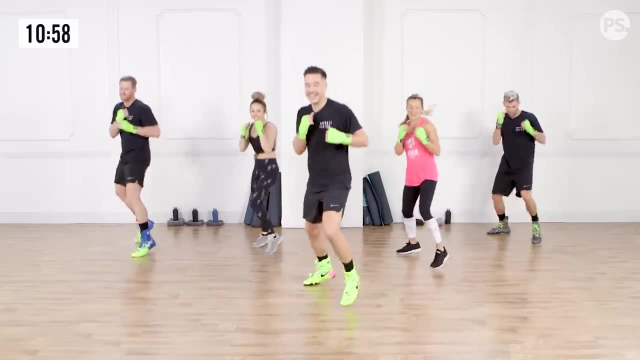 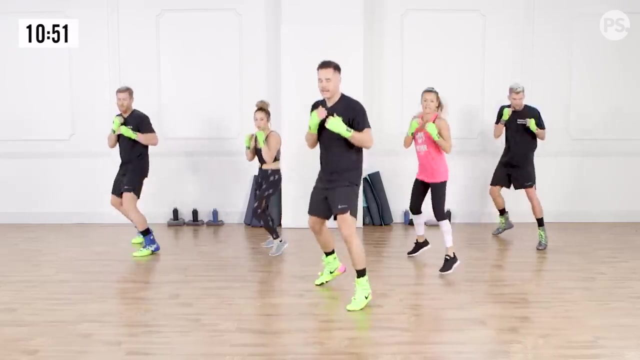 Forward and back, Keeping the hands up 50 times. I'm getting pumped. Yeah, There we go. Yeah, You're doing pretty hard core right now. Good, And all these are legitimate, practical boxing skills that can help prepare you, if you want. 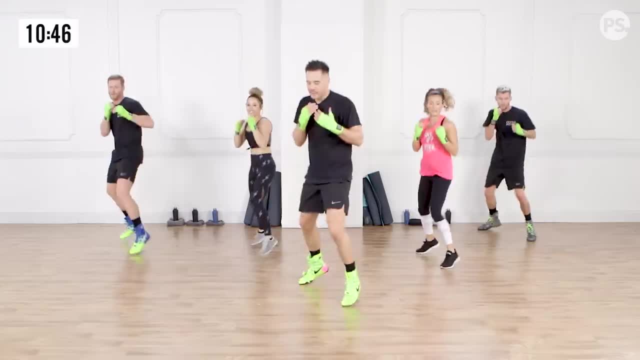 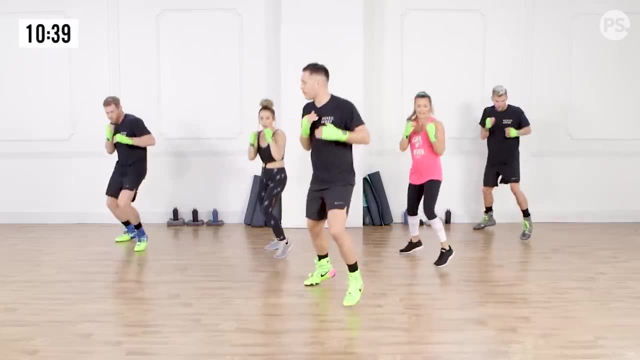 to take your boxing knowledge to the next level. Yeah, All right. So these are great fundamentals. We'll help set you up for success. We got less than 20 seconds left Forward and back Hands up, And if you guys want an extra challenge, you guys can go through this workout a second. 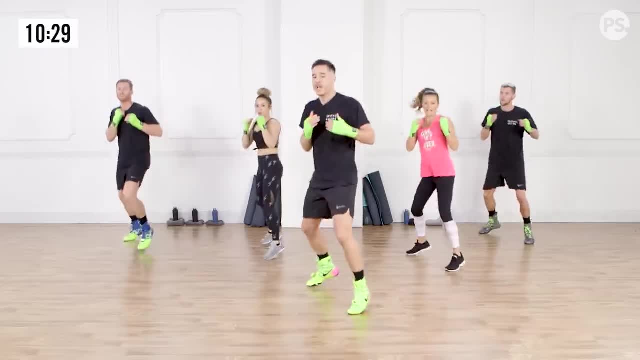 time and work with your right side forward to kind of build coordination, Yeah, On your non-dominant, On your non-dominant side. And if you really really want to take it another step, you can do this workout with hand weights. 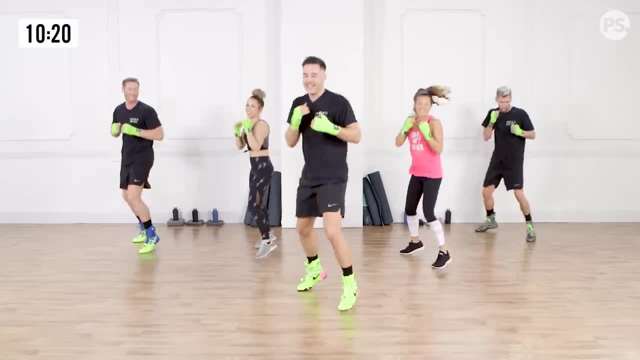 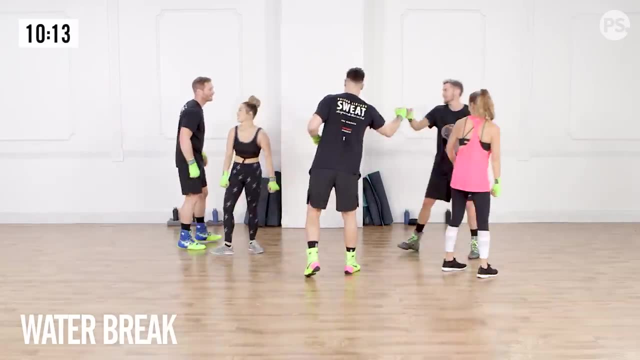 One, two pounds, even five pounds. Oh baby, All right, And break guys. Nice work. That's section two. You guys crushed it. Yes, Good job, Easy, easy, Let's get it. Team, Team talks. 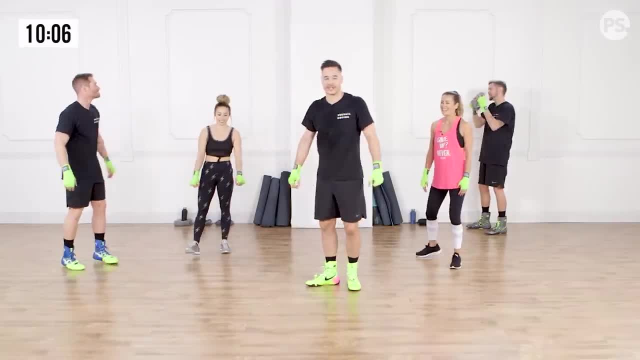 Only got one step left. Uh-oh, Uh-oh. Putting in that work, Putting in that work. It's time to go. All right, guys, For section number three. we're going to be going over. We're going to cover uppercuts and weaves. 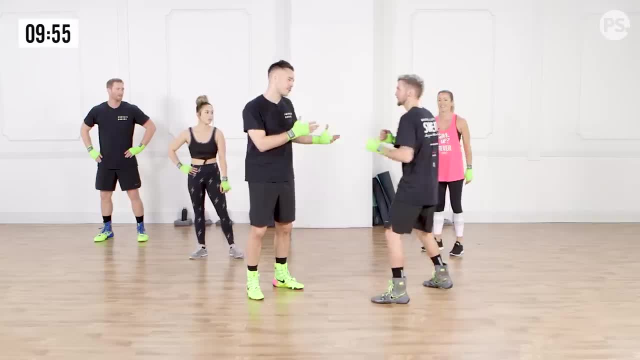 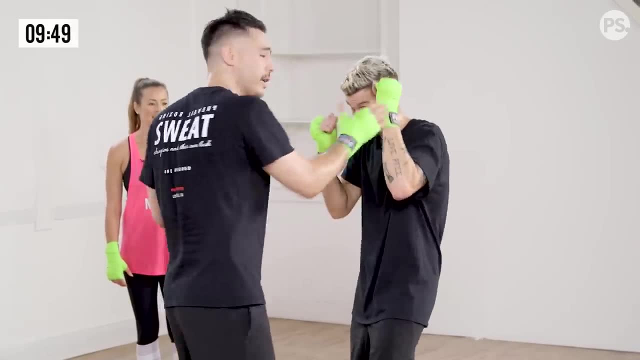 So, Coach Lowe, will you come up? Coach Lowe, First we're going to cover when we use the uppercut right. So my opponent, if they put their hands up like this, maybe the straight punches aren't working. they're ready on the side so I can't throw my hooks. 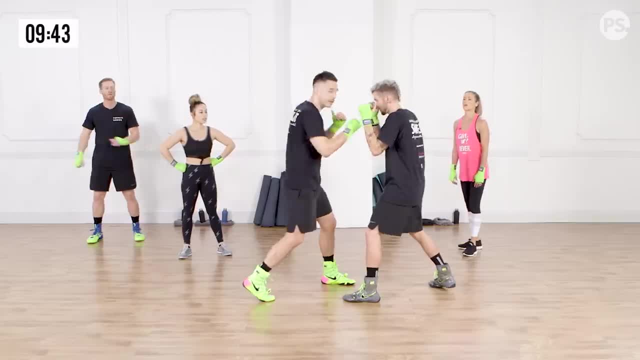 I'm going to go straight up the middle and that's where we use the uppercut. All right, So when I throw my uppercut, a couple details. I'm going to rotate my fist, so my palm is facing me and you'll notice that my elbow 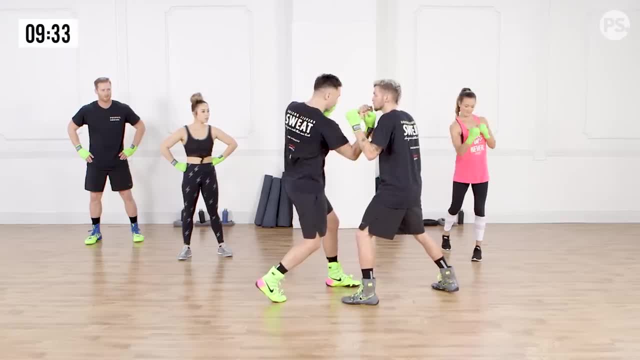 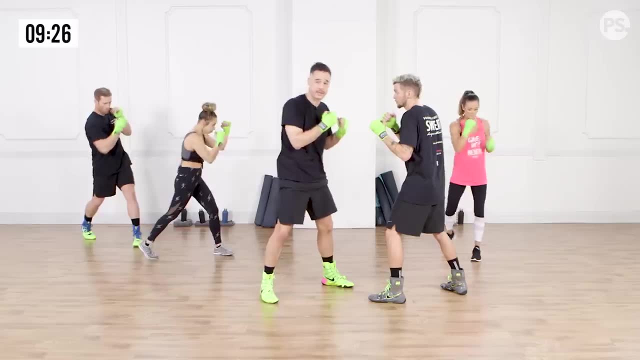 and my fist are in alignment. Okay, I want to come straight up the middle and then reset. Pivoting the hips, rotating the shoulders, Boom and boom. Those are my uppercuts. The other element that we're going to be working right now is the weave. 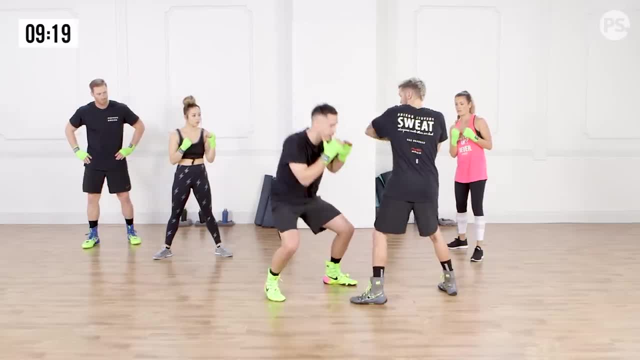 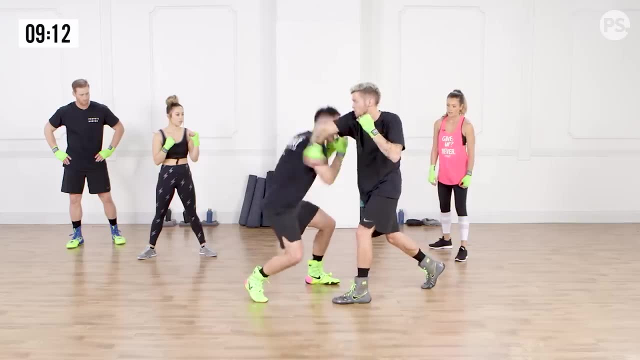 So if Lawrence throws his left hook at me, I'm going to scoop underneath, making him miss, keeping my eyes up and seeing if I've got a punch or if another punch is coming at me and I've got to weave the other direction and throw my punches from there. 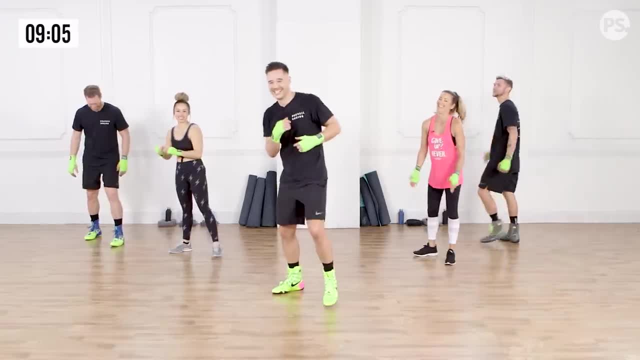 All right, Thanks, Coach. You're welcome, Coach, Thank you, Thank you, Thank you. So from here, we're in a good boxing stance And then we're going to add our bounce. We're going forward and back. 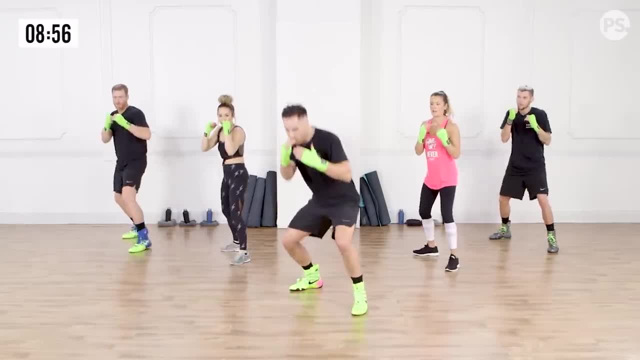 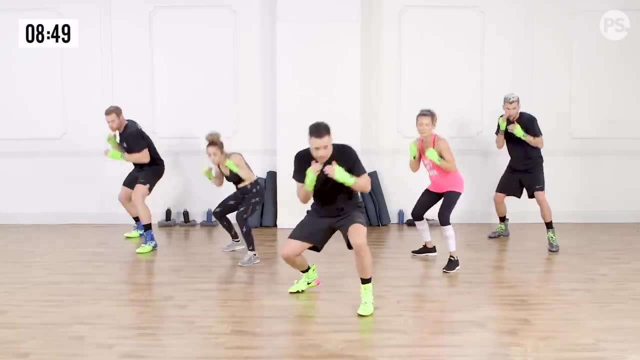 All right, First, when I say go, we're going to plant our feet and we're going to weave and weave. All right, Ready, We're bouncing and we're going to weave to our right, to our left, back to the bounce. 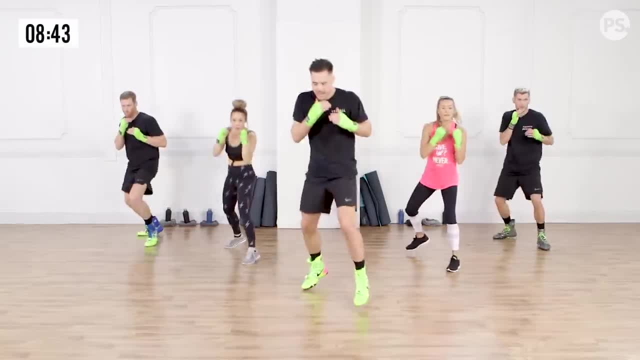 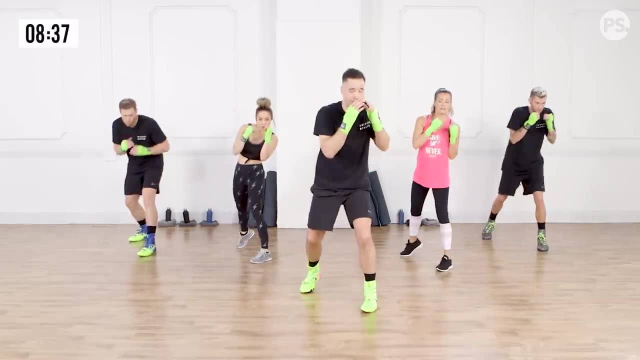 Ready And go To the right and to the left and bounce. So to simplify the movement that we're doing, we're just making a big U with our head going to the right, to the left, trying to stay as balanced as we can. 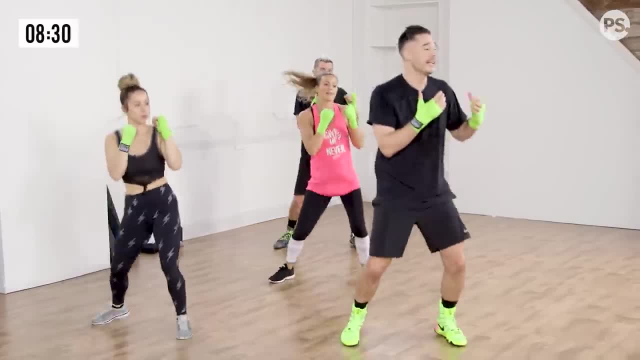 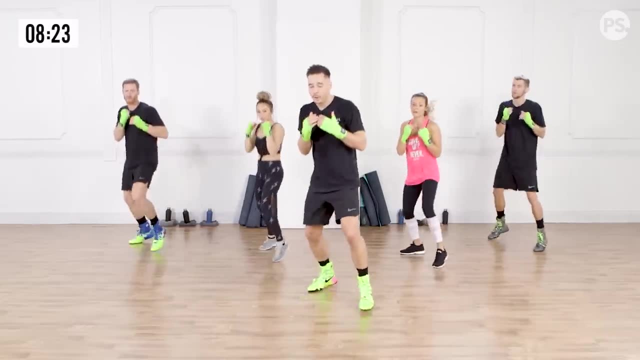 Because from that balance, Because from this movement, we're creating an opportunity to counterpunch And go To the right, to the left. So now we're going to add the punches. when I say go, We're going to weave to our right, to our left. 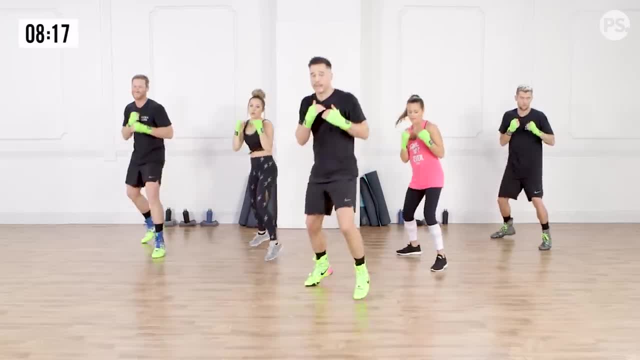 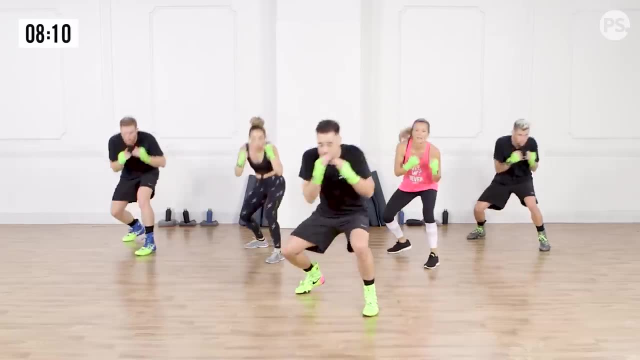 We're going to throw our left uppercut and right uppercut back to our bounce. All right, I hear you guys breathing back there. Yeah, It's a good thing. Yeah, All right, Ready Go, Weave to your right, to your left, uppercut, uppercut. 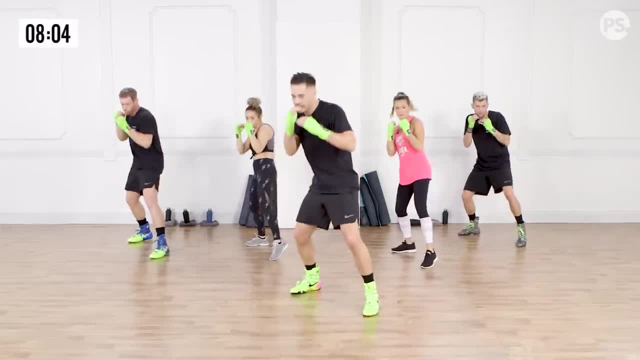 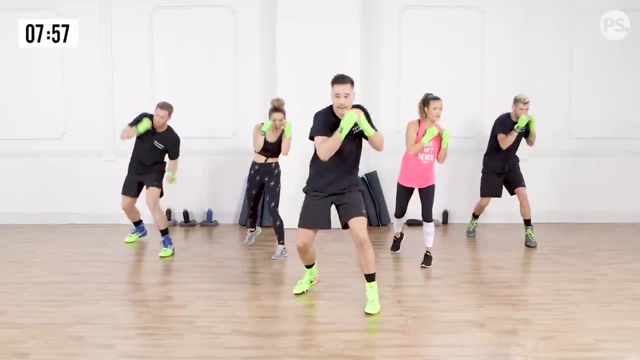 Good, Exhale back there And go. Weave to your right to your left. Hop, hop Right back to the bounce And go To your right to your left. Hop, hop, Good And go. 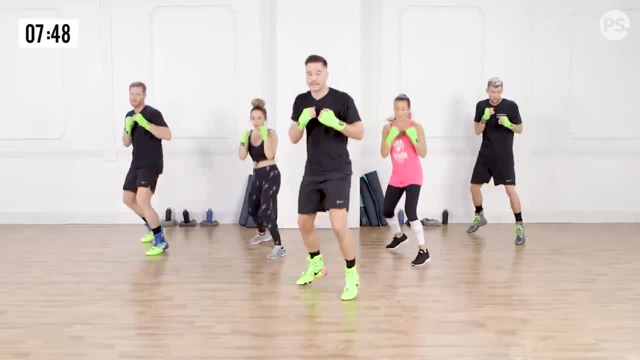 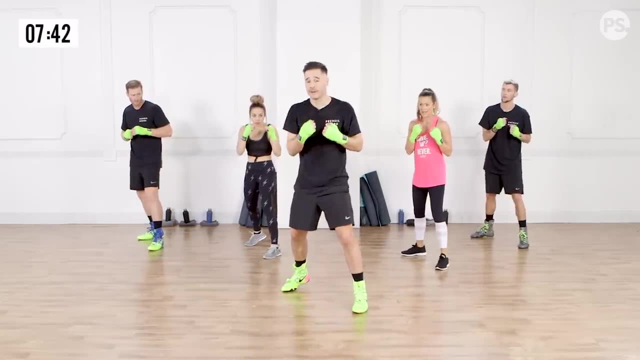 Right, left, bomb, bomb. Good guys, Now this time, whatever number I call out, I want you guys to have your feet planted for this one. You're going to throw that number of uppercuts. So if I say two left, right, 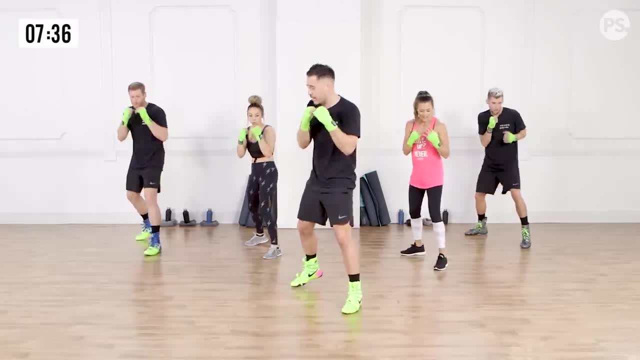 If I say four, left right, left right, All right, Everybody understand. Let's go. All right, Let's get this Ready. Two hop, hop. Remember we're going to start with the left hand first for this one. 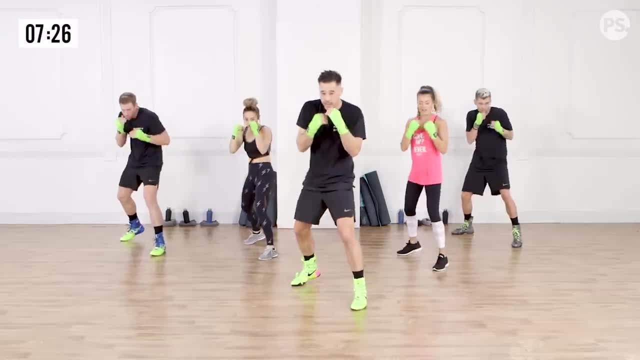 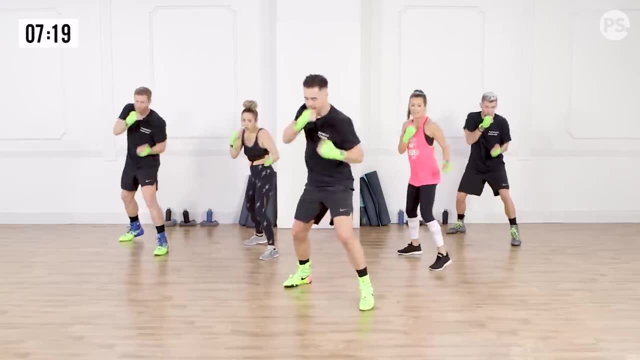 And six: Hop, hop, hop, hop, hop, hop Good. And four: Boom, boom, hop, hop, hop Good. Two Hop hop, Two, Hop hop Ten Woo, All right. 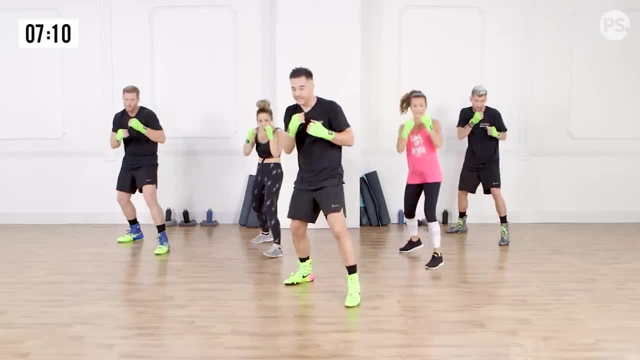 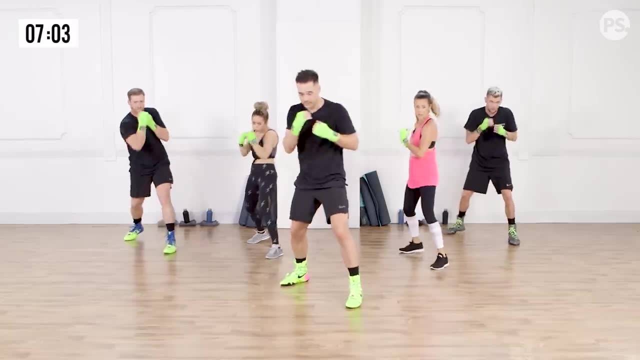 Two Hop hop, Two Hop hop. If I say one, it's just going to be the left Ready. One Hop, Two Hop hop. One Hop, Three Hop hop, hop Good. 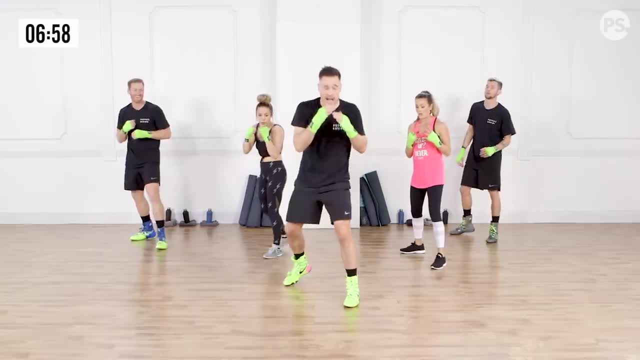 All right, guys. Now we're going to add the weave to it. So, whatever number I count, I want a weave to the right, to the left, and that number of uppercuts. All right, Let's go, Let's get it. 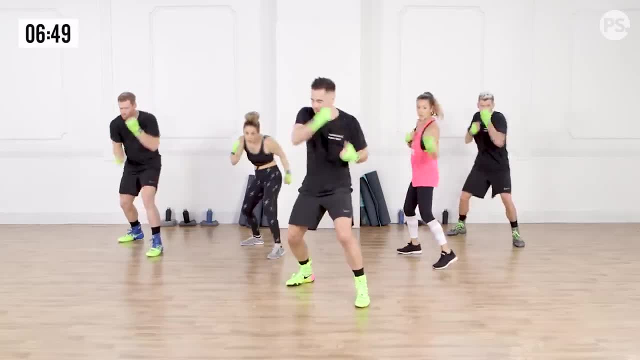 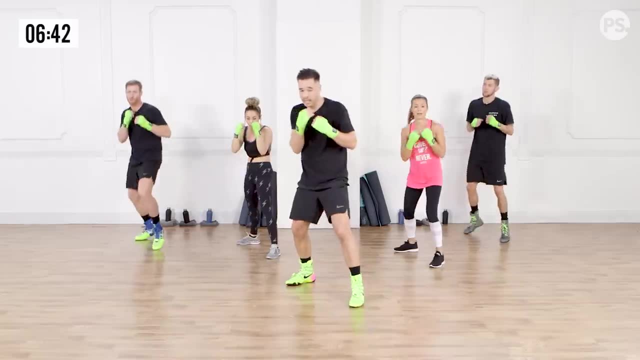 Ready And two Weave to your right, to your left, Bam bam, Good Four To the right, to the left. Hop, hop, hop, hop, Coming straight up the middle, right past our chin, and focusing on the recoil down. 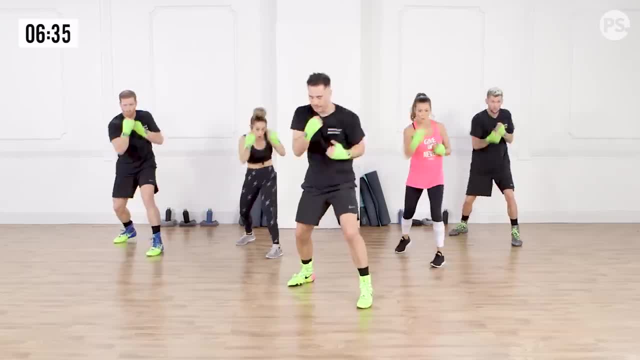 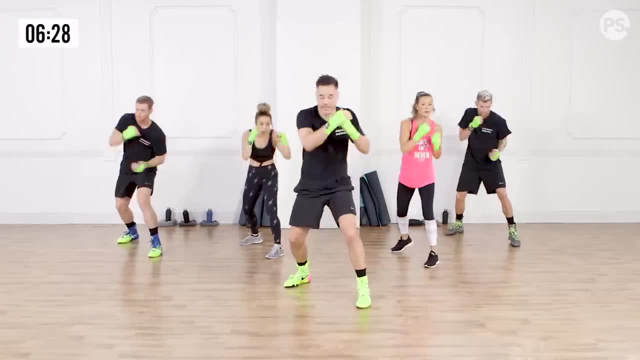 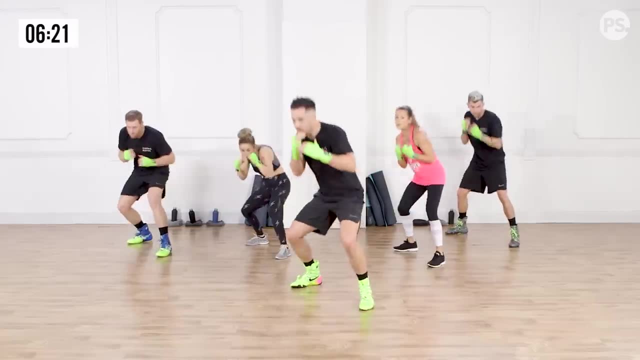 One, two Good Six. Right left, Two Hop hop. Good. Go, Two Hop hop. One Weave to your right, to your left, Left, uppercut, Good, All right guys. 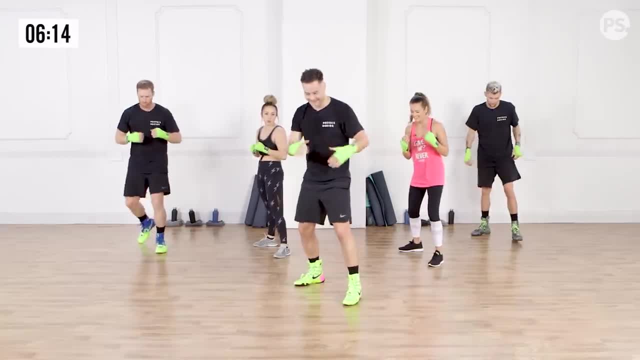 We're going to go 30-second shoe shine challenge. What that means is we're going to plant our feet, We're going to go as fast as we can with these uppercuts and we're going to give it all. we got 30 seconds. 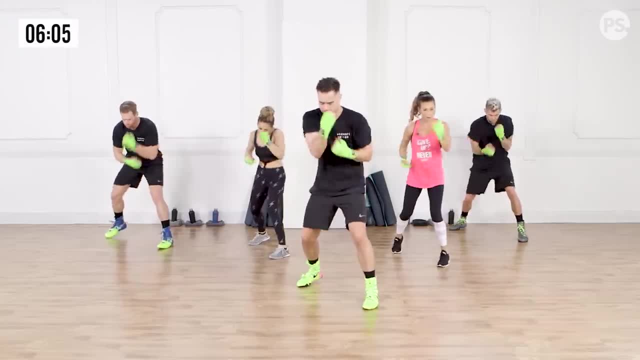 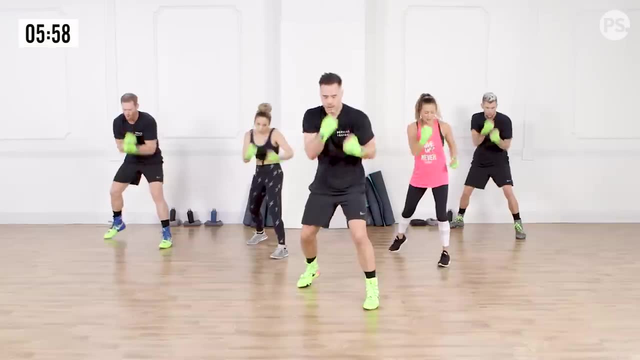 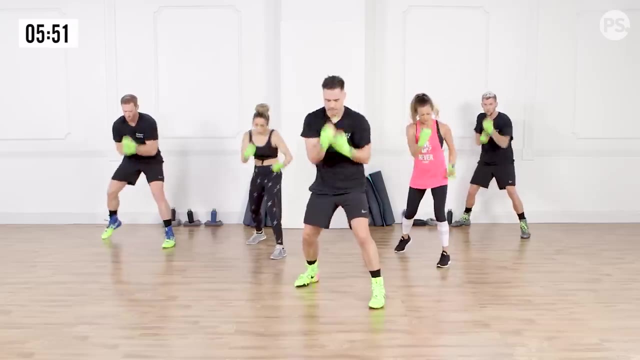 Going in Three, Two, One Shoe. shine, Remember, we're going to come all the way up. We're going past our chin Core's engaged, Feeling it coach, Yeah, Come on, Come on, Remember, speed kills. 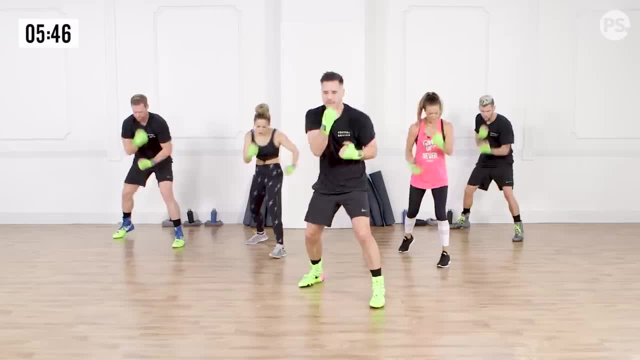 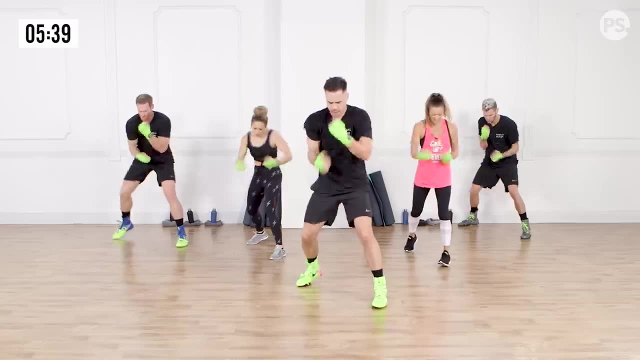 All right, so that's what we're working on here. Everybody's tired, but champions push through that tiredness. right, We get to the next level: Five seconds. I want you to go as fast as you can right here. One, two, three, two and one. 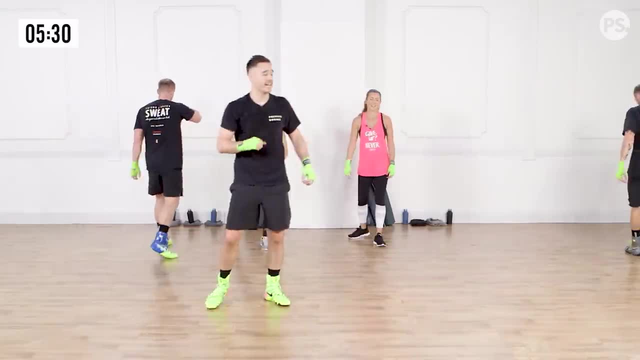 Nice work, guys. Burn it Good job, Good job. Go ahead and grab a mat. I didn't think it was going to be that tiring. Let's grab a mat. Finish with a little bit of core work, Okay. 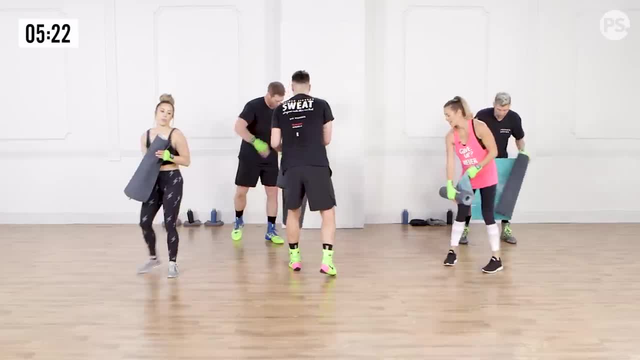 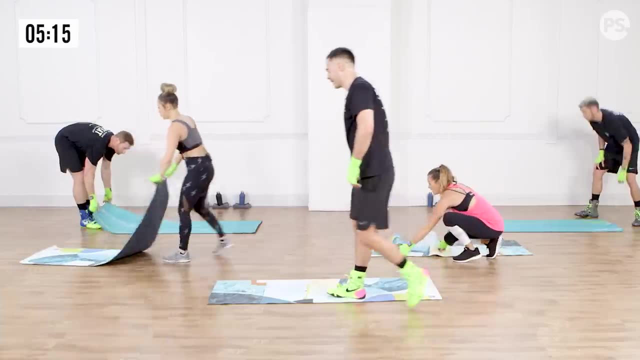 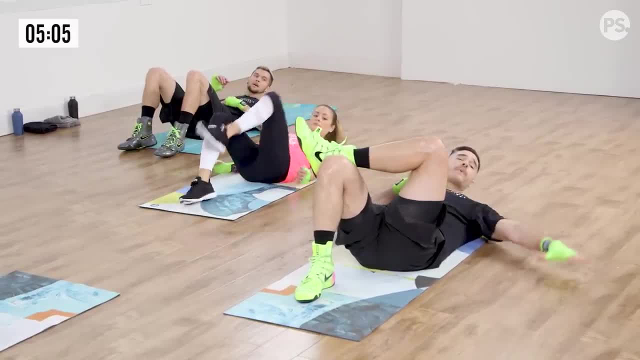 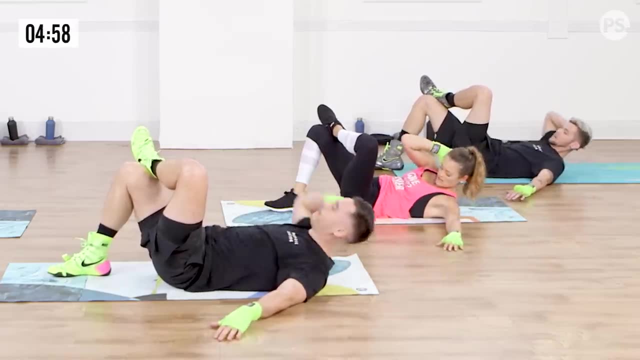 Let's cross our left ankle over our right knee. We're going to put our left hand out. We're doing crossover crunches. Bring our right elbow to our left knee for 30 seconds, Big twist. Try and connect the two if you can. 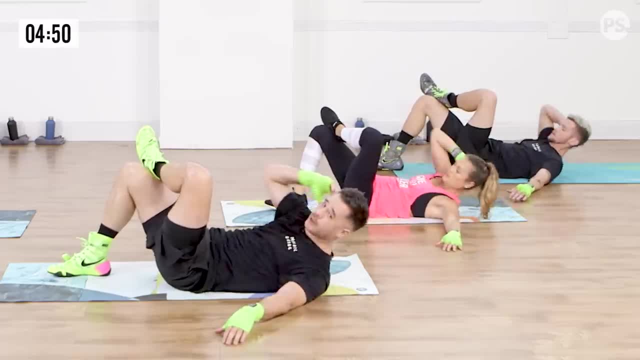 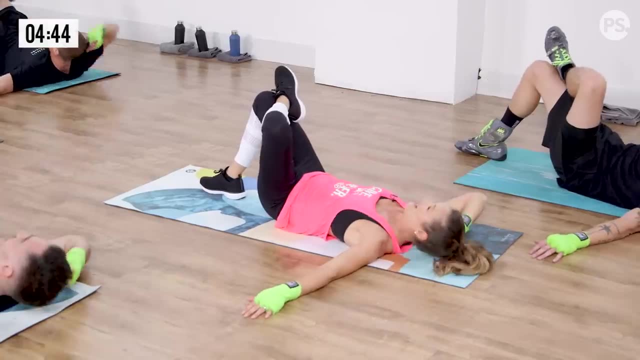 Exhaling on your way up. Very good, Ooh, really trying to connect to it, Push me to that next level. I was taking it easy at first. There we go. That makes a difference. It does, And this is how we develop that rotational power for our punches. 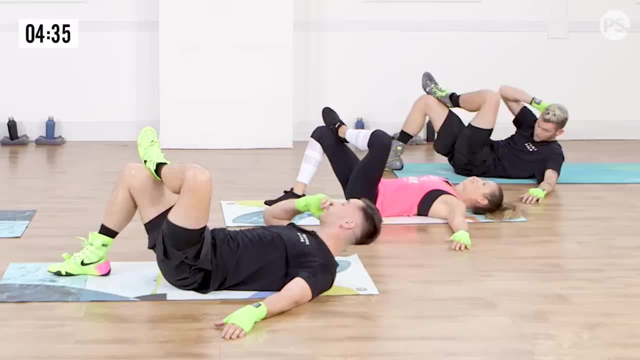 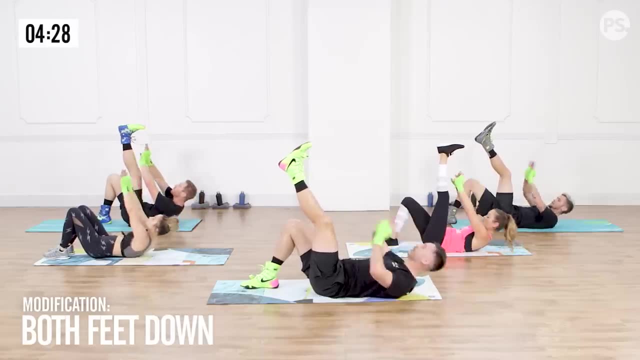 Yeah. So if you want a real knockout punch, you need a strong core. All right From here, guys, we're going to lift our left leg straight up, taking both hands and reaching up for our toe. All right For 30 seconds. 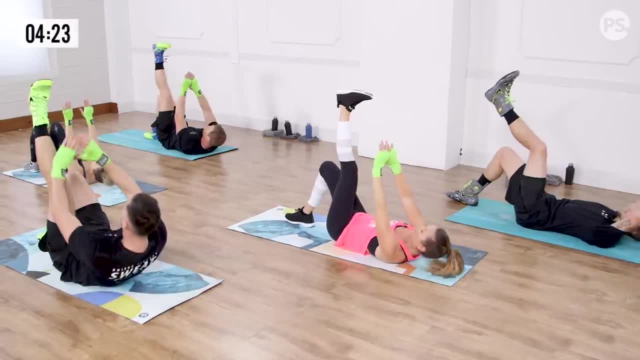 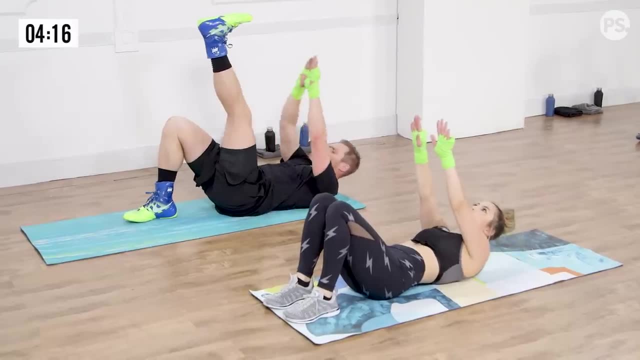 Nice controlled movement. Try not to jerk too much Exhale on the way up And, for a modification, you can have both feet down on the ground like Leilani's doing- Perfectly. Very nice Breathing Exhale. 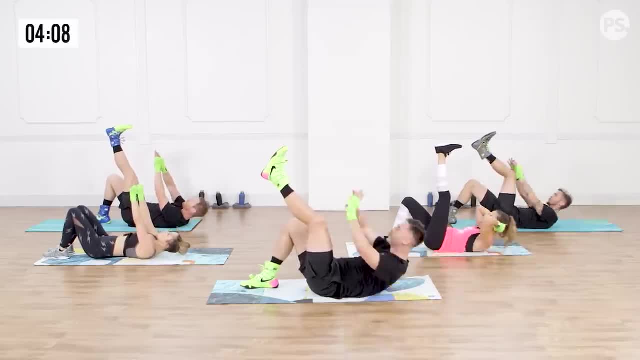 And in three, two, one, We're going to cross our right ankle over our left knee. All right Right hand goes to the ground And again we're trying to connect elbow to knee for 30 seconds. Guys are doing awesome. 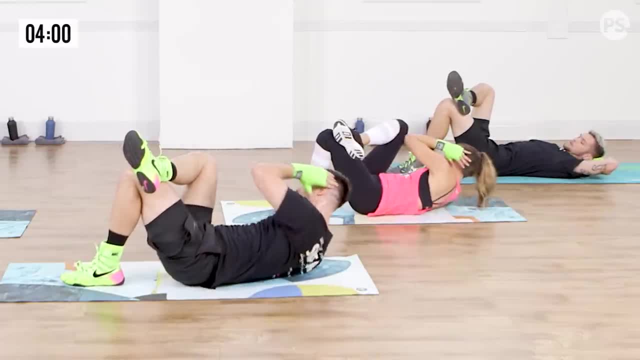 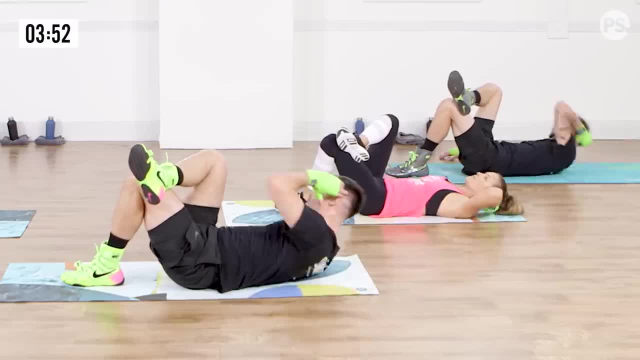 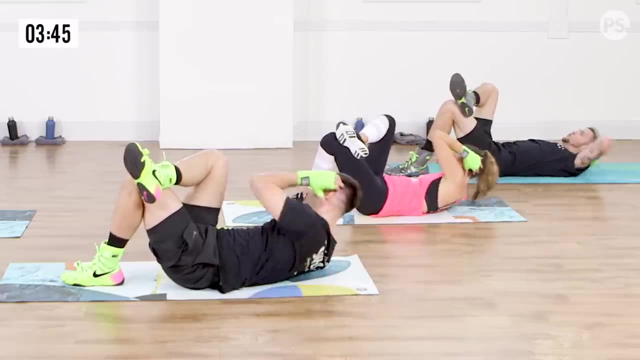 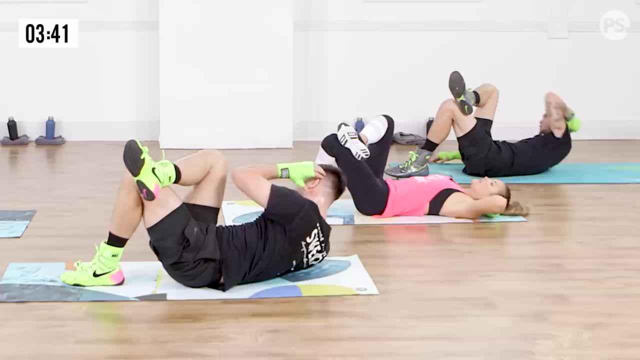 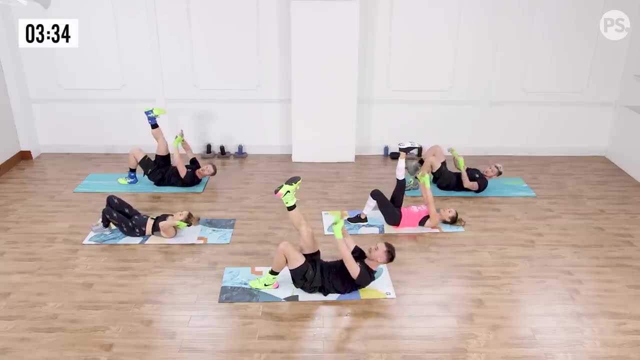 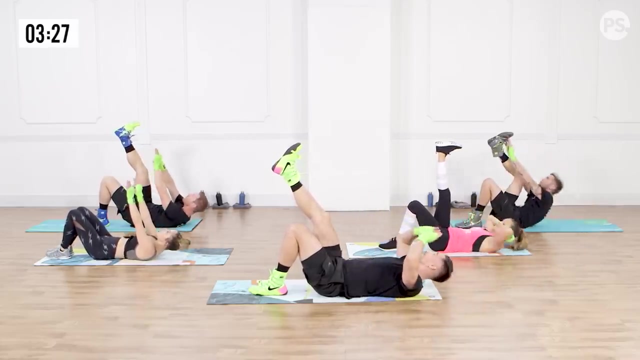 Let's kick it ourselves for greatness, for our best. all right, good. now from here, right legs gonna extend straight up, reaching up with both hands, exhaling on the way up, and I tend to support my neck here because I start to feel it. but great modification, I'm trying not to cheat. great modification if you guys are. 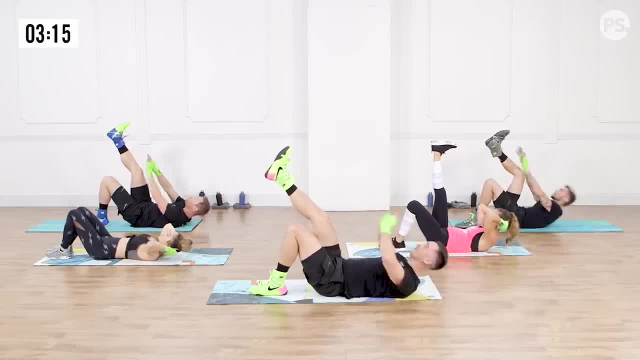 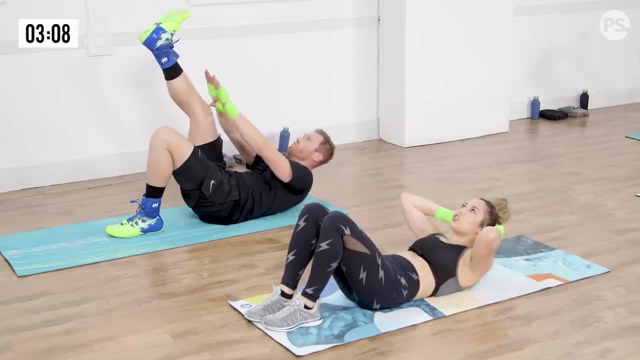 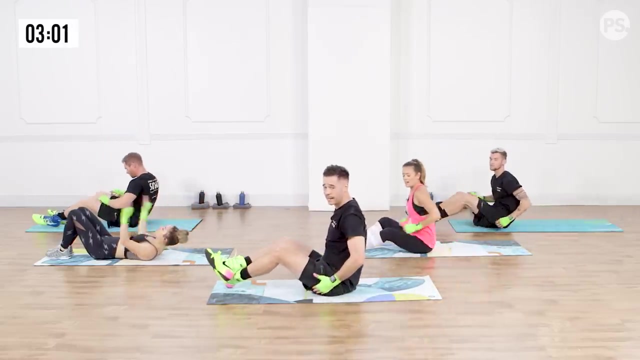 feeling it in your neck back home, feel free to do the same as Anna. if you're not feeling it, a good thing to do is just keep your eyes focused on the ceiling and try to focus on coming straight up. good, good, now, from here, guys, we're gonna do oblique twist. so for the oblique twist, we're balancing on our 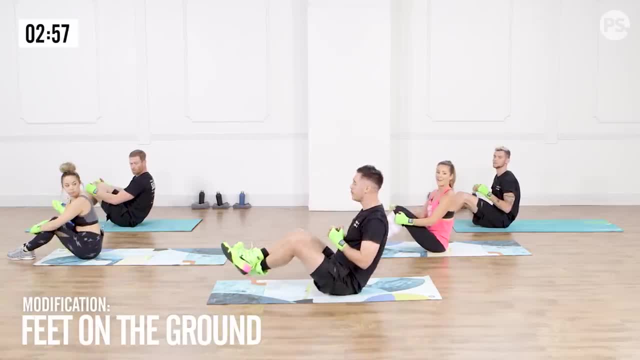 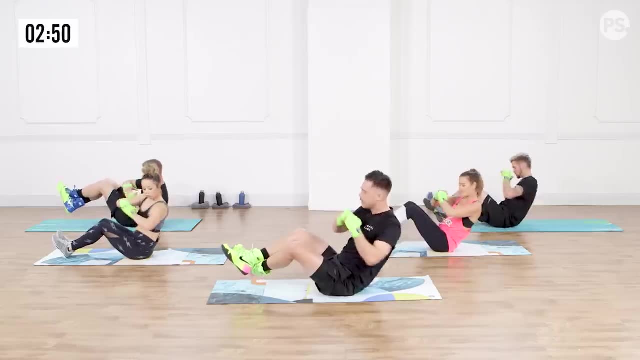 butt, you can have your feet on the ground, but if you want an extra challenge, you're gonna pick your feet up. your hands are in front of your chest and we're twisting from side to side. try to keep your hands in front of your chest the whole time. that way, the range of motion is contingent upon the twist. 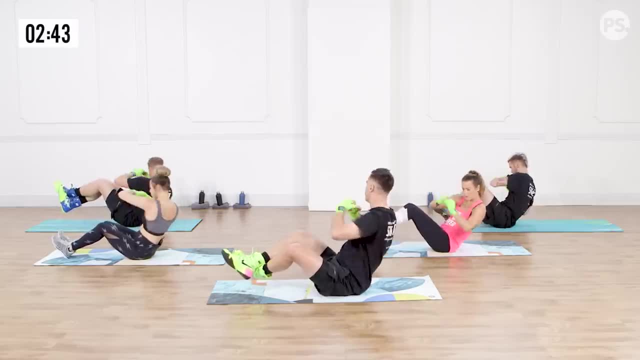 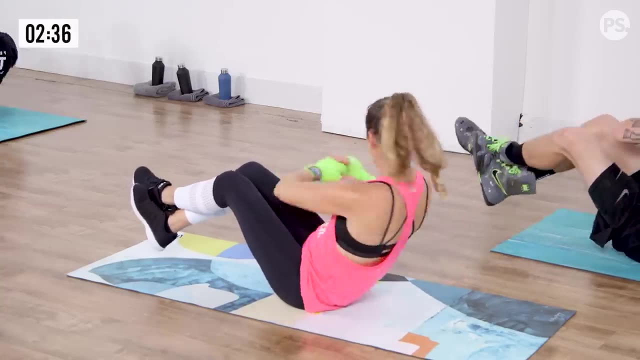 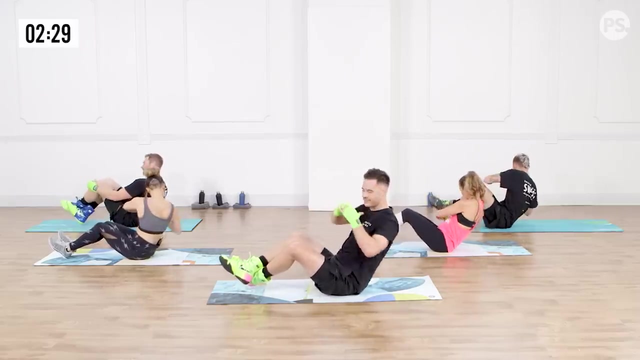 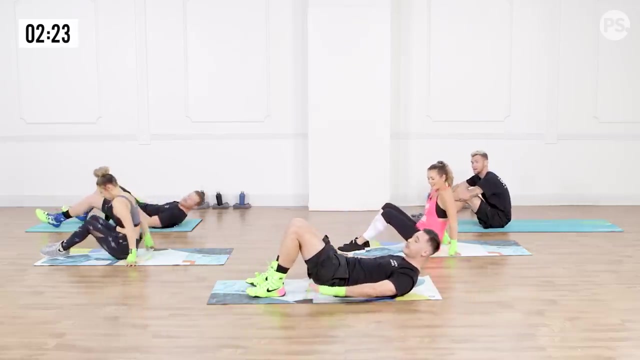 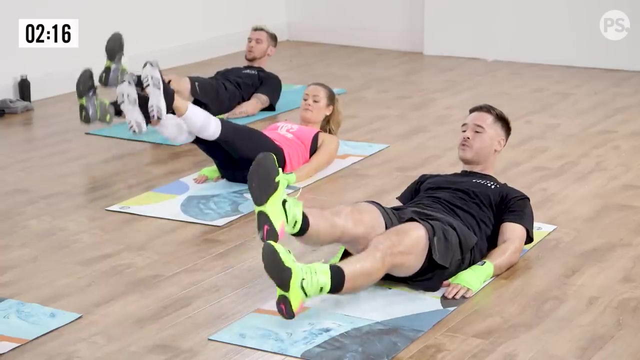 through your trunk. all right, nice to see you there. now let's get this crazy control that's coming right. with this제가 against today, we're gonna take the force of the time itself and make it our star again. this is how we're developing our rotational power for power punches. I feel that, yeah, oh, my goodness, this is a good one. Coach Lowe, what do you always say? of course, Strong, Money Long. baby k Ps. We're strong and Money Long. lets get paid now. from here, guys, we're gonna go Flutter Kicks right here or, if you need the hands, Continue videos and follow us. 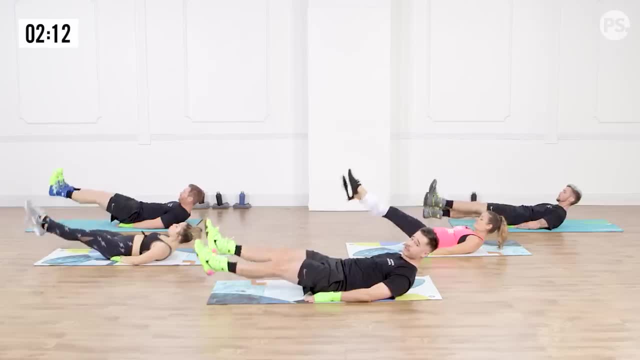 small range of motion, keeping your head and your shoulder blades off the ground. Good, We're going to switch the jackknives in three, two, one. So for the jackknives, I'm coming up, I'm going to slap the mat, bring my knees to the chest. 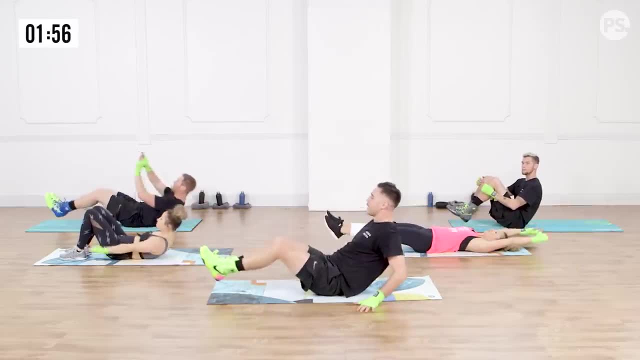 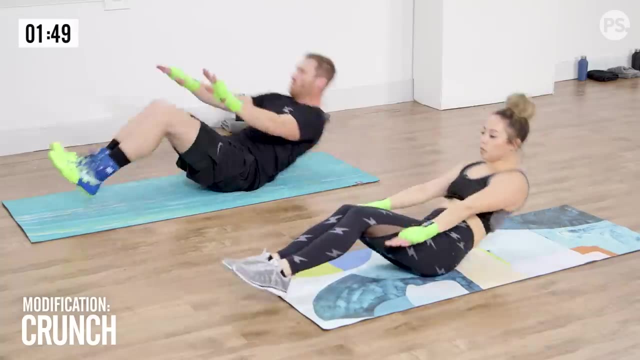 boom For modification, so you guys can put your hands out to the side and you can just bring your knees to chest. all right, So you can go here. or you can go crunches, as Leilani's doing, for a simpler version, all right. So again, we can extend out like this: 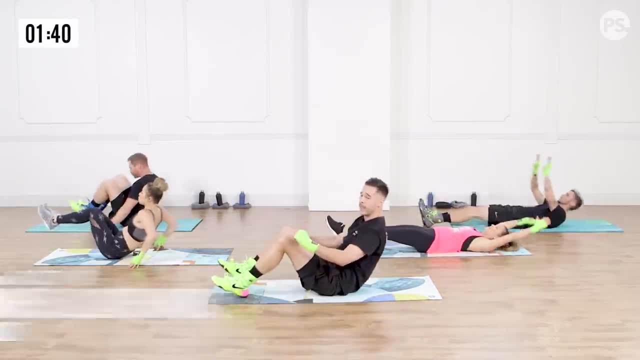 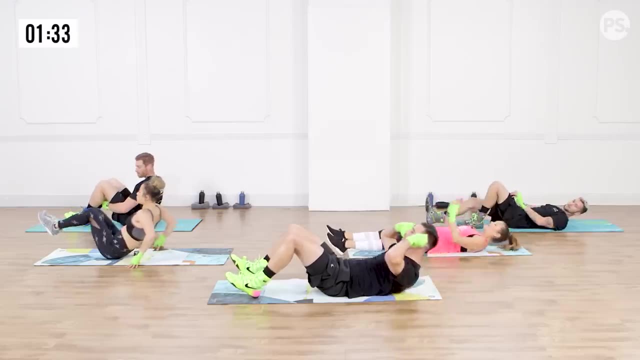 or we can just do crunches, or we can come all the way up slapping the mat. all right, Good. And from here we're going to switch to mountain climbers in three, two and one. So everyone flip over. We're going to be in a push-up position, bringing the knees. 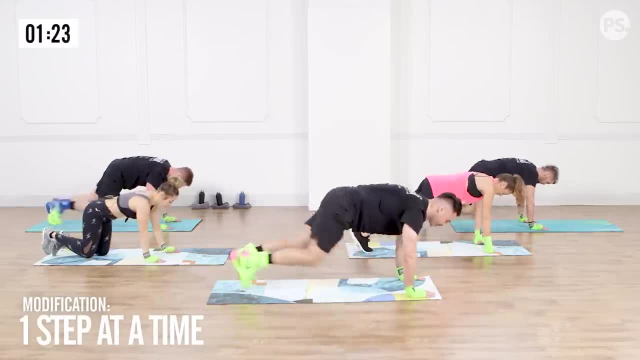 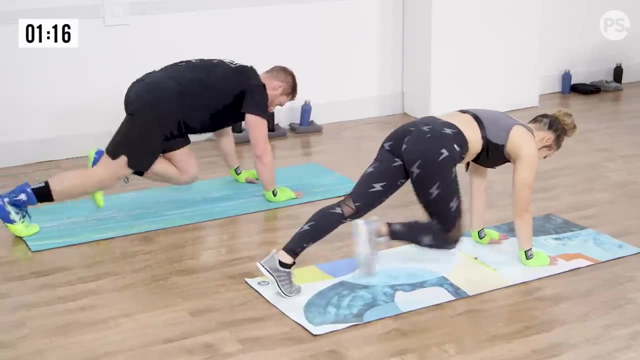 up towards the chest. okay, So we're here trying to run up the mountain or, for a modification, you guys can step like Leilani's, doing one foot at a time. Good, Ten more seconds. Let's sprint up that mountain. Yes, get to the top, baby. 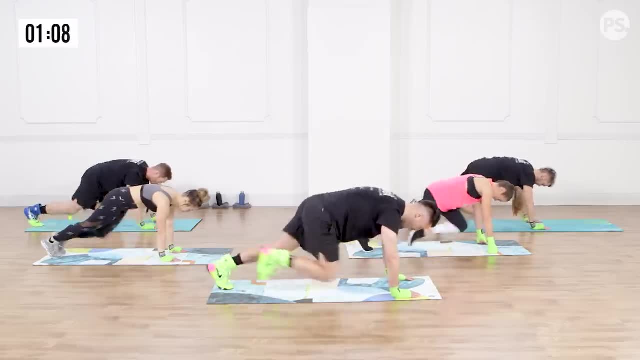 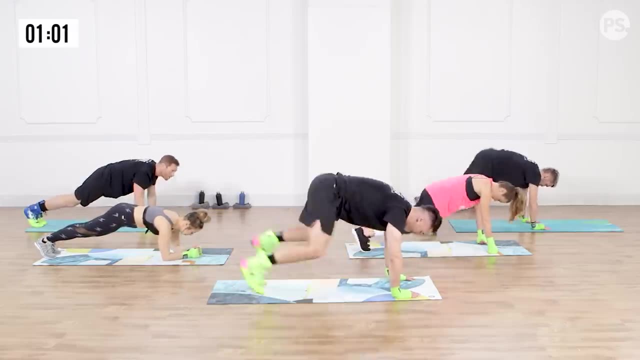 On that mountain. Turn up Three, two and one Four-point plank jack. So we're going to go open up back and close. Oh my gosh, Open up back and close, And if you guys need a modification, you can just hold a plank from here. 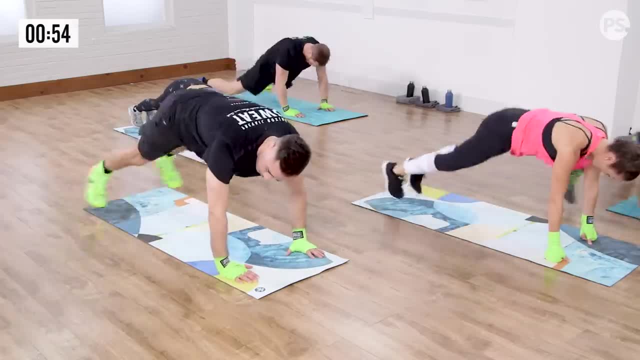 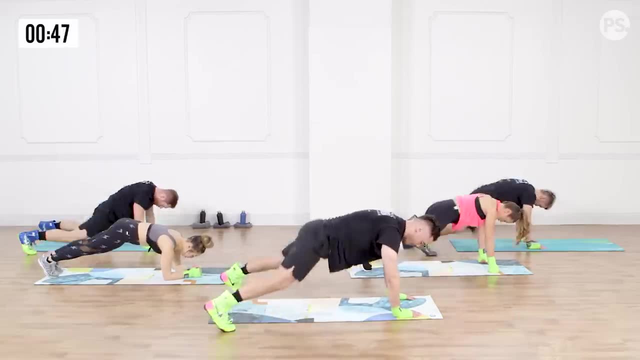 back nice and flat Boom. Oh my gosh. Yeah, these are great. huh, This is awesome. This is awesome. I like this move. All right, we're going to go to an inchworm with a knee tuck in three. 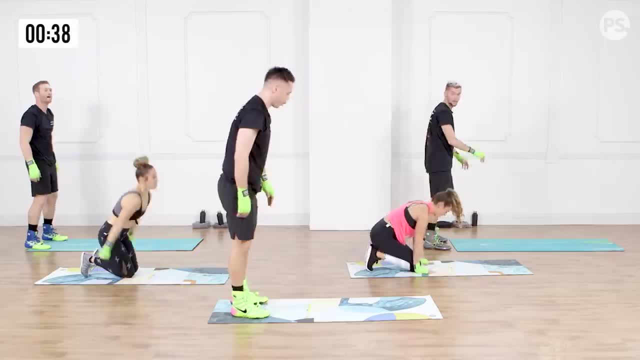 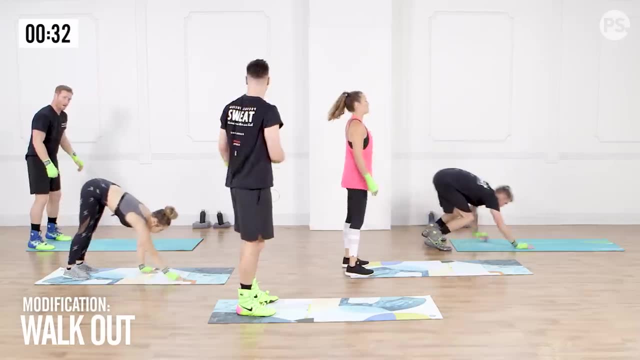 two and one From here. guys, we're standing up, We're going to walk our hands out, nice and fast. walk them back and knee tuck. Oh, baby, For a slight modification, take out the knee tuck. All right, guys, 30 seconds, Let's get it. 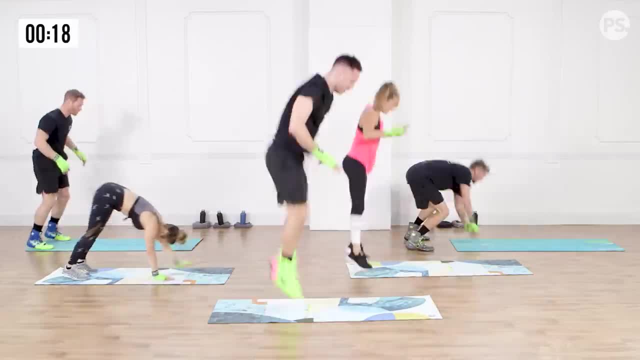 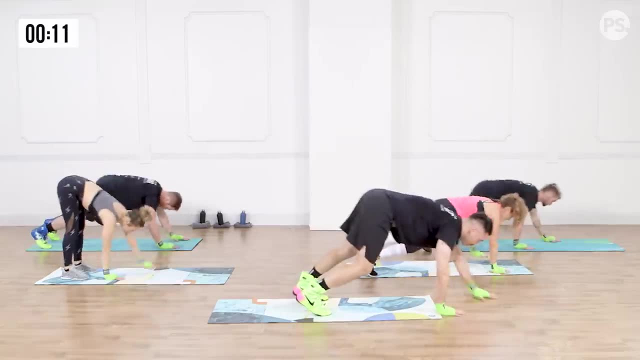 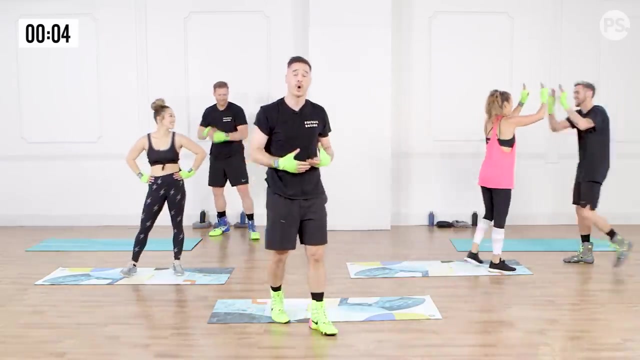 All right, Doing good. 10 more seconds, Three, two and one. All right, guys, Great job. That's a wrap for the workout From here, guys, we're going to go ahead and stretch it out. cool down When you guys crush it. 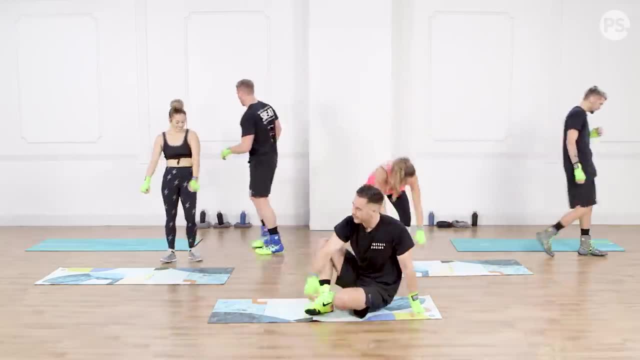 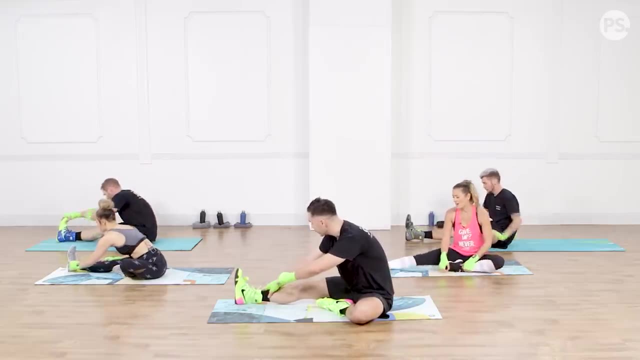 Thank you. Hey Loni, Thank you. I'm sorry We're going to start off figure-four. stretch Right leg out, Left leg in, hinging from the hips, reaching with both hands for your toes, if you can, oh we're. 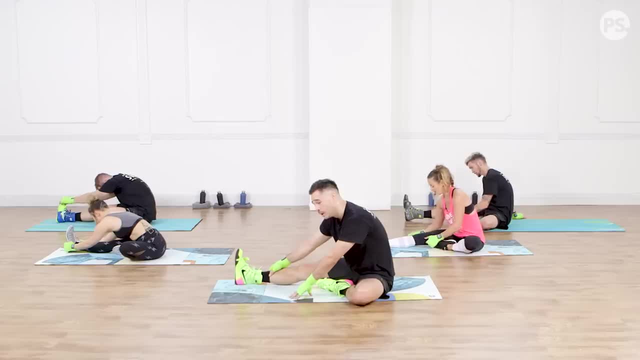 just gonna hold this for about 30 seconds. a nice static stretch. I'll show the modified version of this, Thank you, The unflexible version. Make sure that you guys are breathing. it's a good hamstring stretch. yeah, okay if I bend my knee a little bit. yeah, if you need to. 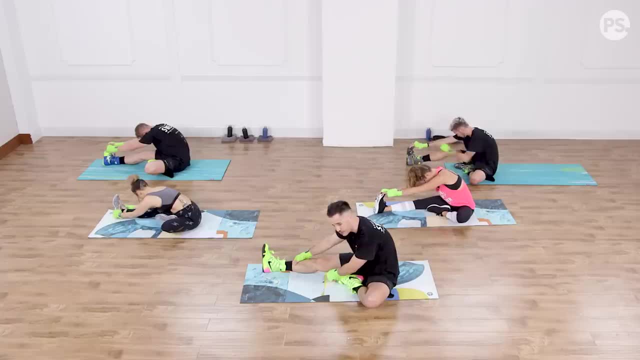 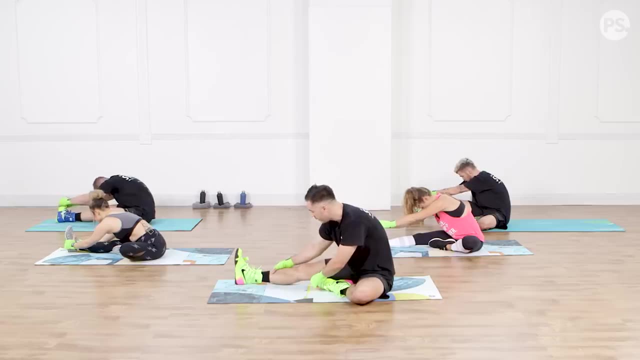 bend your knee a little bit, it's totally fine. again, this is just you versus you, all right. so, wherever you're at at home, just trying to push a little bit further than what you're comfortable with, nothing more than that, and let's go ahead and switch. so now we're gonna have our left leg out, our right leg folded in. 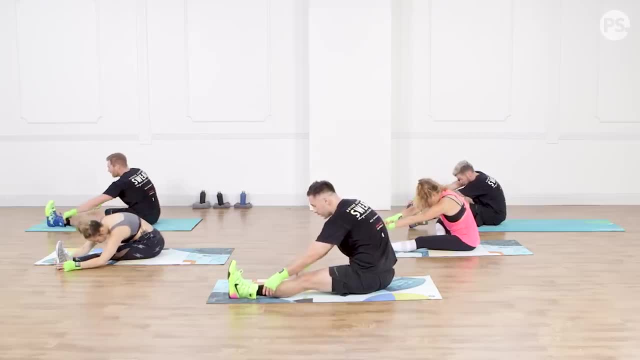 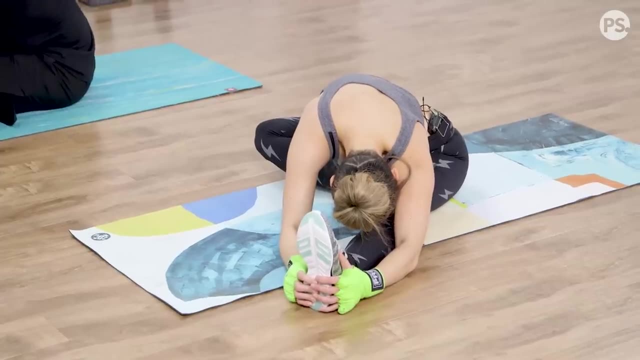 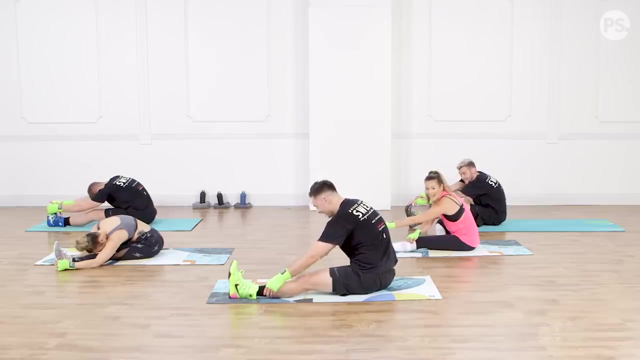 and reaching out with both hands for me. I'm just going for my ankle. even that's challenging, but as you can see, Leilani's gone past the foot down to the heel- yeah, head to knee. one day I hope to be on her level. We all aspire. I will be there one day. 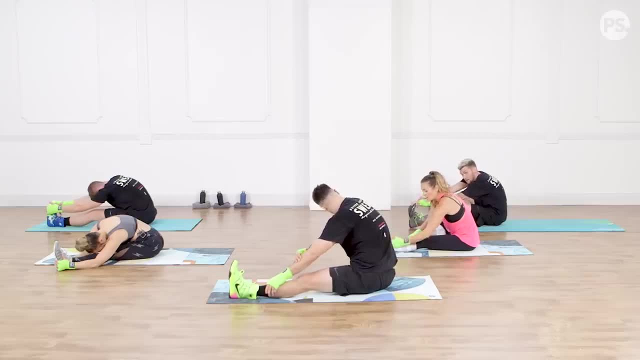 Yeah, I love how that workout was such a good mix of learning some real quality boxing moves and stances with the conditioning, so that was such a great combo- Awesome, thank you. yeah, that's, that's totally the goal. all right, let's go ahead and have. 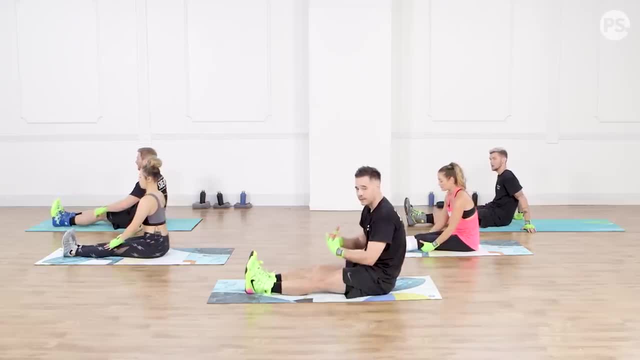 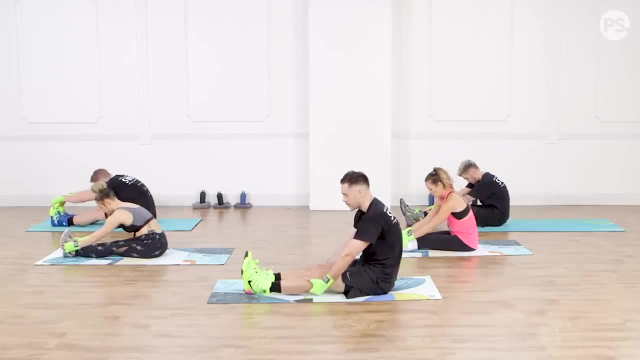 both legs straight out in front of us. I find personally that when I'm learning a skill set while working out, it makes it a lot more enjoyable and more fulfilling for me personally. so hopefully you guys enjoyed it at home, learned some new stuff, got a good start, Yeah. 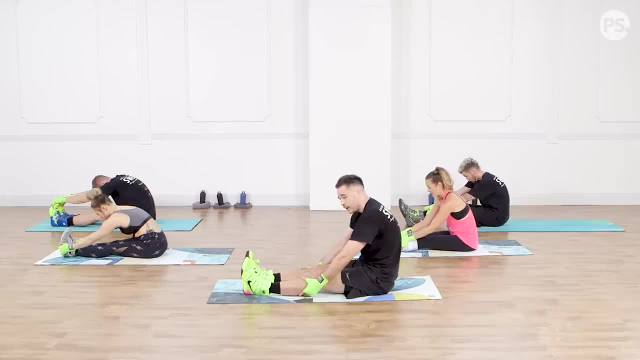 Had a good sweat, like we all did, and hopefully you'll do this workout again with us. Yeah, and when you go to boxing classes, you won't feel as coordinated when you're practicing the basics, Absolutely. so you know, this is a great thing to do, maybe before you take that first boxing class or if you're just 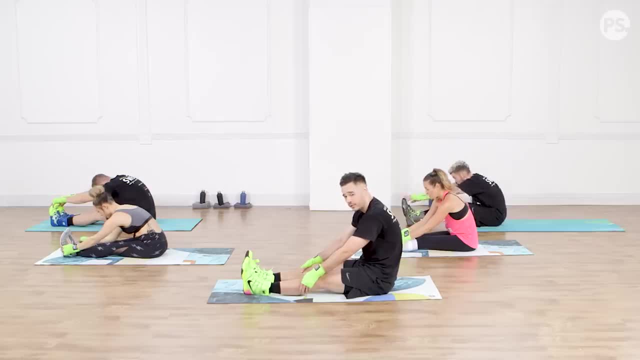 trying to polish up on you know something, getting some that ring rust off, just drilling the fundamentals, getting comfortable with these intense little sprints and then short recoveries, because that's really the pacing of real boxing. Yeah, All right, Excellent work, guys. We're going to go ahead and get started.